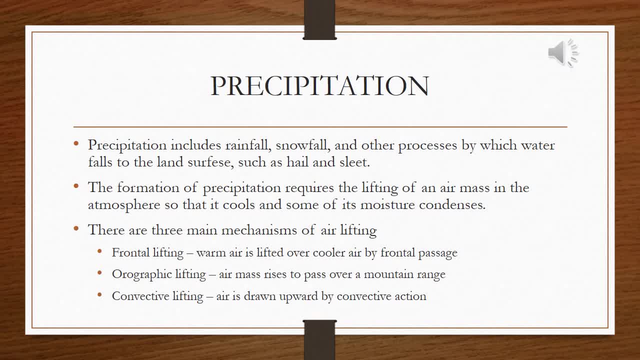 First part is precipitation. Precipitation includes rainfall, snowfall and other processes by which water falls to the land surface, such as hail and slit. The formation of precipitation requires the lifting of an air mass in the atmosphere so that it cools and some of its moisture condenses. 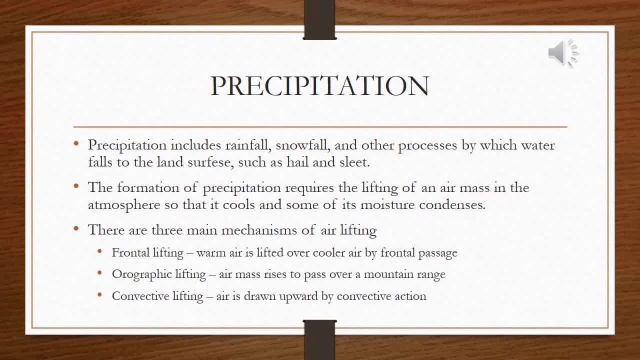 There are three main mechanism of precipitation. The main mechanism of air lifting: Frontal lifting, orographic lifting and convective lifting. Frontal lifting: warm air is lifted over cooler air by frontal passage. Orographic lifting is air mass rises to pass over a mountain range. 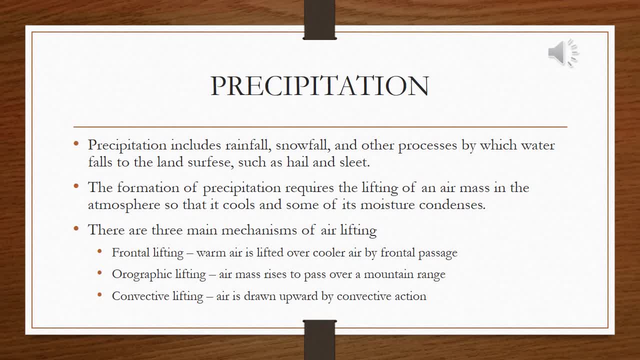 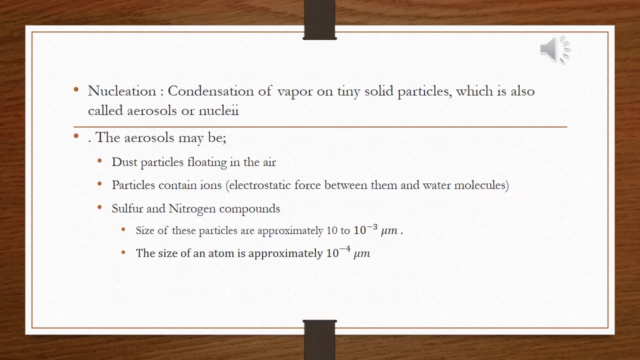 And convective lifting is air is drawn upward by convective action. All this was covered in hydrologic class last year detailed, So I'm just going to remind you of this one as precipitation. In order to precipitate this moisture air, it's just not enough to have the meeting this warm air or air moisture. 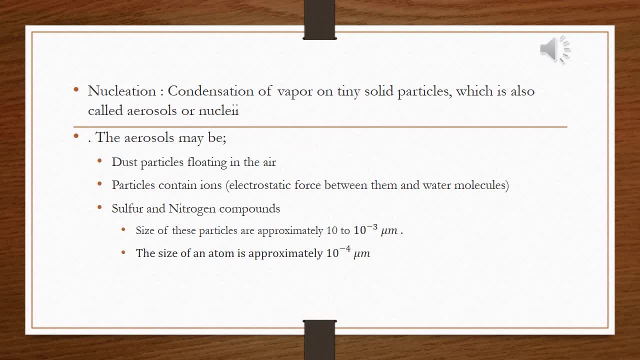 And it's also necessary to have a process called nucleation, which is condensation of vapor on tiny solid particles, which is also called aerosols or nuclei. So it also needs these air molecules or water molecules need to meet with this tiny solid particles, Which are they. 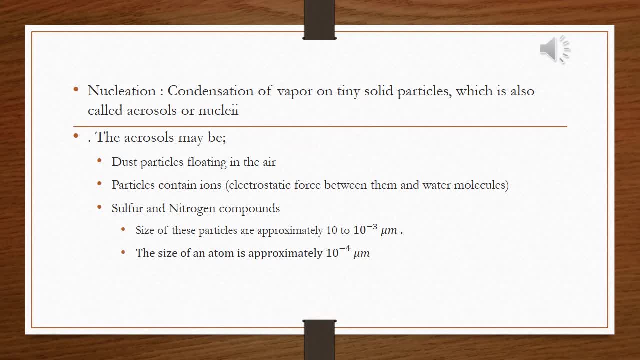 The aerosols may be dust particles floating in the air. Particles contain ions like electrostatic force between them and water molecules, or like sulfur and nitrogen compounds. This sulfur and nitrogen compounds is from the combustion, from the industrial stuff. It's going through the air. 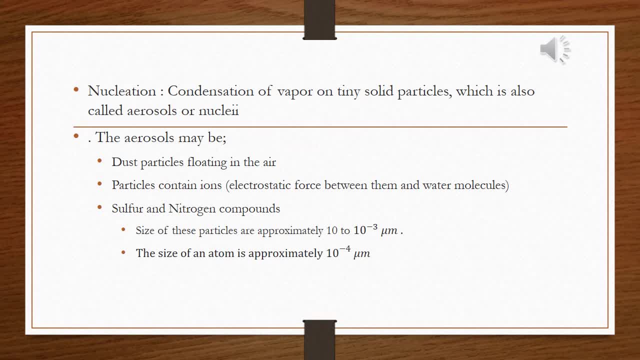 If we look at the size of these particles, this aerosols, is between the 10 to 10 to minus 3 power power 10 to minus 3 micrometers. The size of these particles- And in order to compare this one we can also see the size of item- is also approximately 10 to minus 4 micrometer. 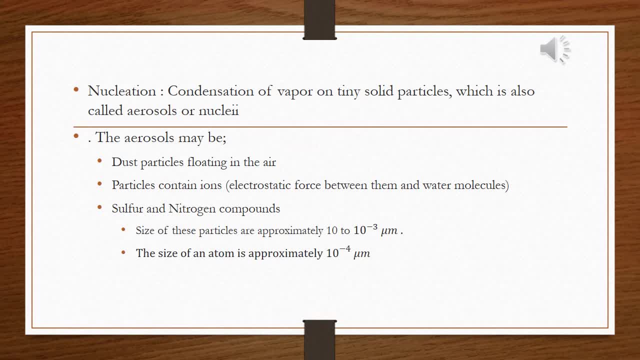 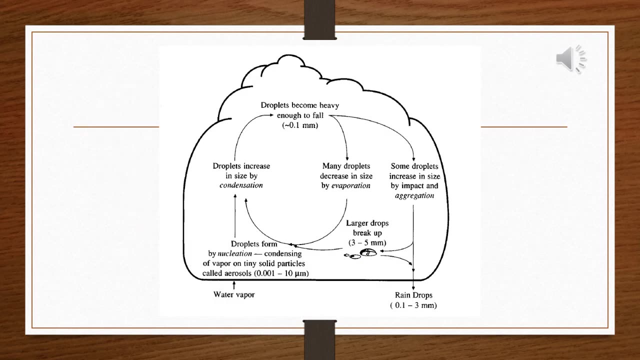 So that's why, like I'm giving you, like it's going to be maybe like 10 times atom Size or like a thousand times of atom size of these aerosols, And this is the graphical representation of rainfall or precipitation. First the water vapor goes up with evaporation and then droplets form by nucleation. 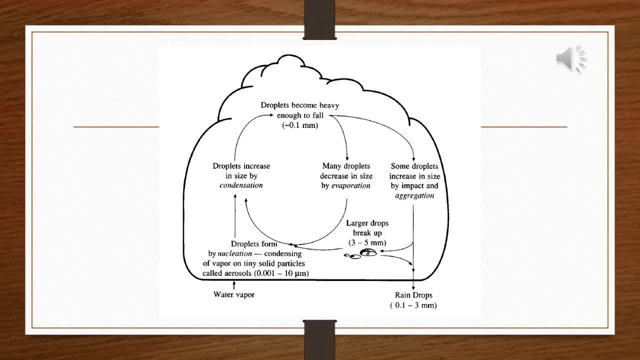 So it's going to be a form of droplet. Condensing of vapor on tiny solid particles is aerosols, What I gave you just right now, which is like 0.001 to 10 micrometer. Then it goes up to droplets, increase in size by condensation. 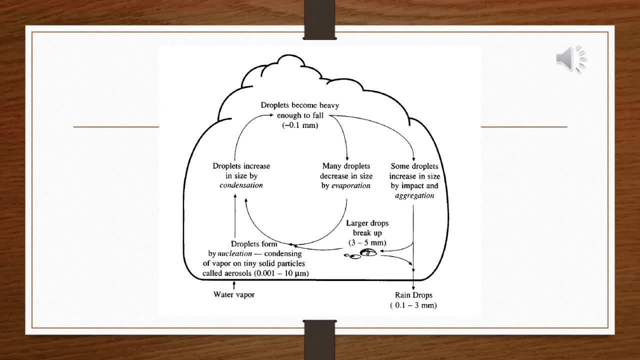 Okay, And by time is again going up. by forming a cloud, The droplets becomes heavy enough to fall, which is going to be like 0.1 millimeter, from 0.001 or 10 micrometer to 0.1 millimeter range. 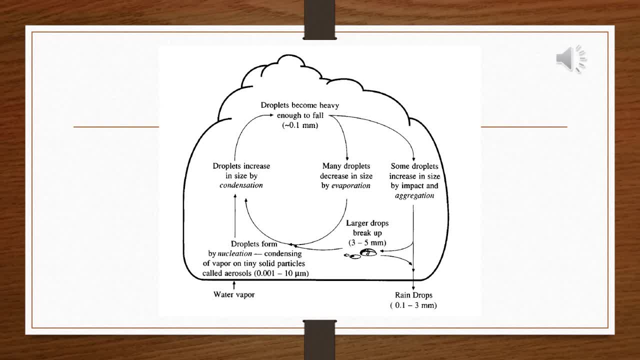 Which is like an around like a thousand times of droplets. Okay, So it's getting like bigger and bigger, Then it gets heavy, Then it start to fall down. Many droplets decrease in size by evaporation, Again, like when it goes down from the atmosphere because of the like the sun's radiation. 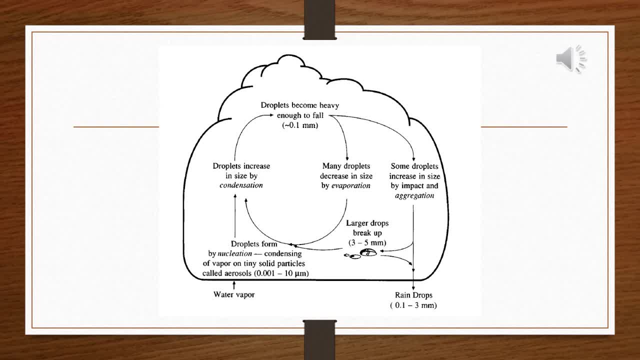 So it increases the like, the thermal reaction with the radiation, and then it decrease the size. So it goes again up on the clouds And some droplets increase in size by impact And aggregation. So when it meets with this droplets and other droplets it gather together. 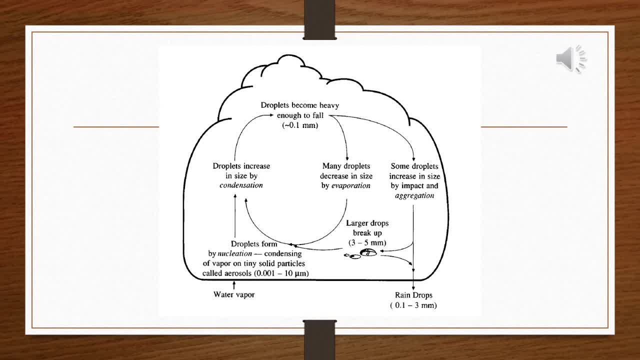 So it aggregate and it start to fall down. But due to the like, the wind power and then the drag forces it larger drops, Maybe the breaks up and then goes again. It gets lighter and it goes again up or it falls down with the this droplets which aggregate and then fall down as a whole. 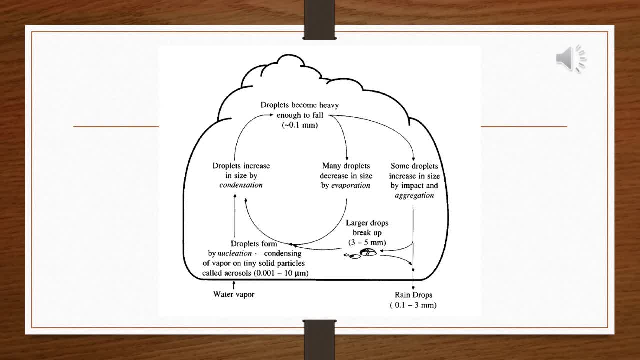 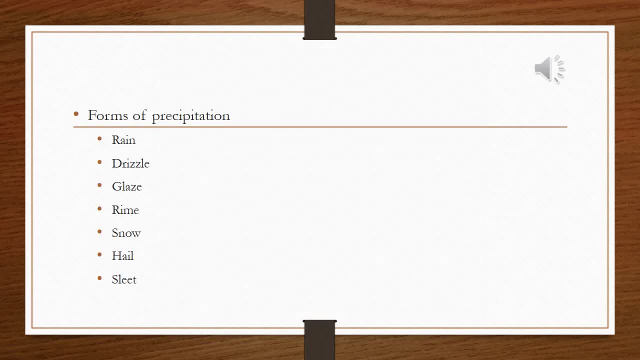 Okay, So we can use the rain drop, which is 0.123 millimeter range. It is good to also touch the form of precipitation. We have several types of precipitation, which is rain first, Then Drizzle, Glaze, Rime, Snow, Hail and Sleet. 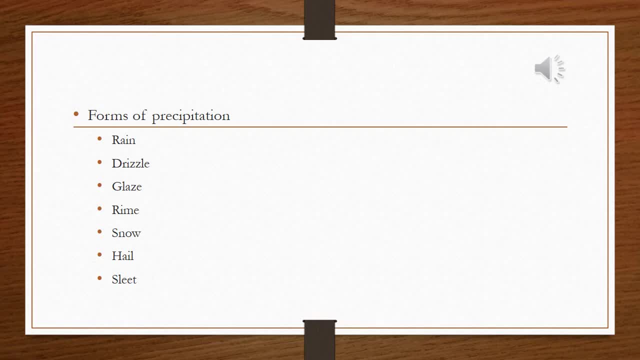 Interesting, Interested students. Students can go through and then see the size of all this precipitation range and See, like, how it forms and what is it. You guys can see it. why we were talking about the precipitation is very important. parameter is One. one of the important parameter parameter is terminal velocity, which is when the rain drop. 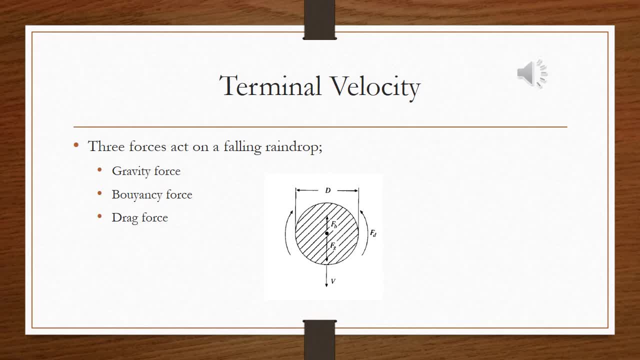 It Starts to drop, like with the terminal velocity, the constant velocity. So how this phenomena occurs, we need to know Which condition effect on it, and then we need to drive the formula to in order to calculate the terminal velocity. Three forces act on a falling wind row: the gravity force, bonus force and drag force. 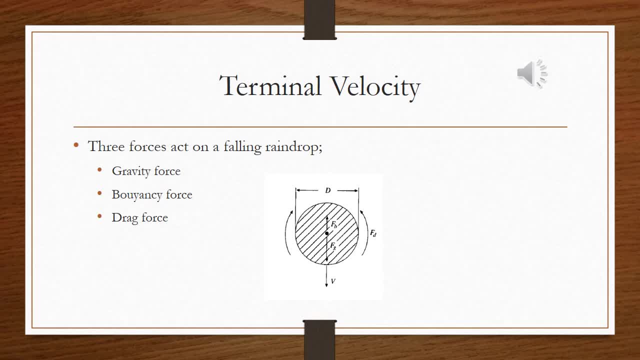 so the when we see here, as you guys see, there is an gravity force is pulling down and Drag force is pulling up and the bonus force, as the moves is downward, is gonna be up. so we know that the gravity force Is gonna be equal to buoyancy force and rain force. 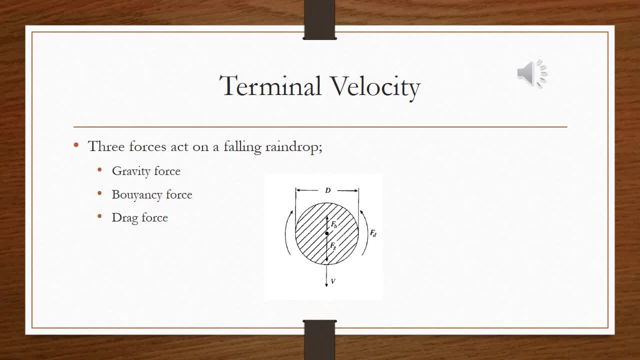 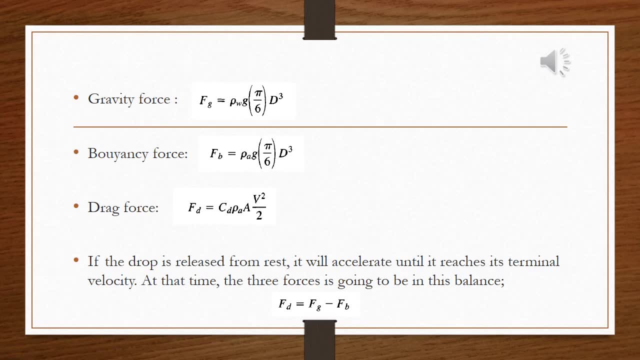 summation. Let's go through the formulation and we are gonna Drive this terminal velocity equation. Gravity force can be represented as the water Density, gravitational acceleration and pi over 6 d-cub, which is the volume, Volume x. the Density is gonna be our mass mass x. gravity is gonna be the force. 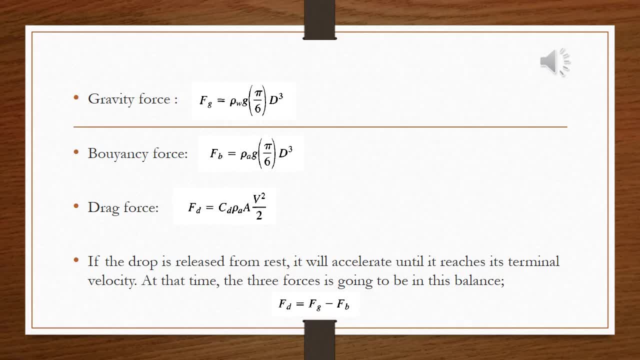 Okay, so it's gonna be the gravity force is representing in this form, is open form of, and buoyancy force is the air is affecting on the, this water particle. so density of air, gravity, pi over six d cube, the then, and this rain drop diameter is uh gonna be our buoyancy force. 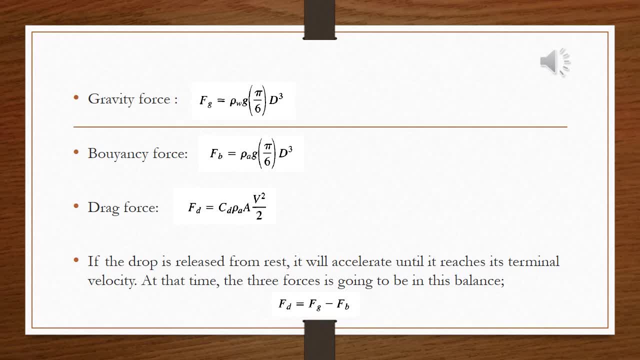 and the last one is the drag force: the, the coefficient of drag multiplied by the air density area of this water particle. the velocity of the velocity square of this particle over two give us the drag force. if the drop is released from rest, it will accelerate until it reaches its terminal velocity. at that time, the three forces is going to be: 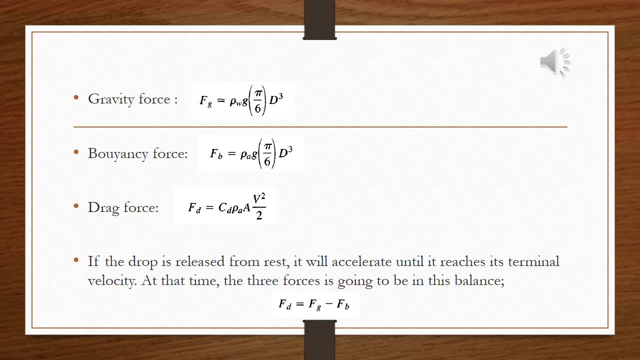 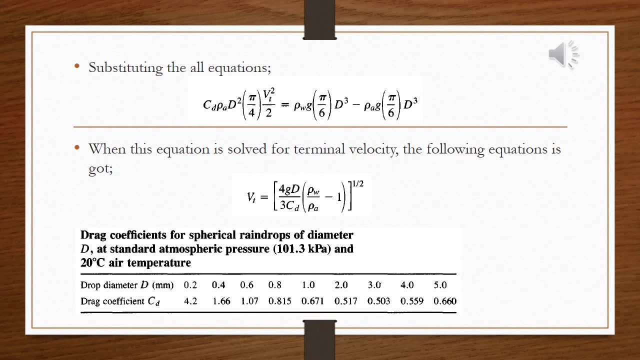 in the. in this balance, which is direct force is equal to gravity minus buoyancy force. okay, when we substitute all the equations in the previous uh equation uh is gonna give, in this form, the, the coefficient of drag. uh, the density of air d square, pi over four v one square. 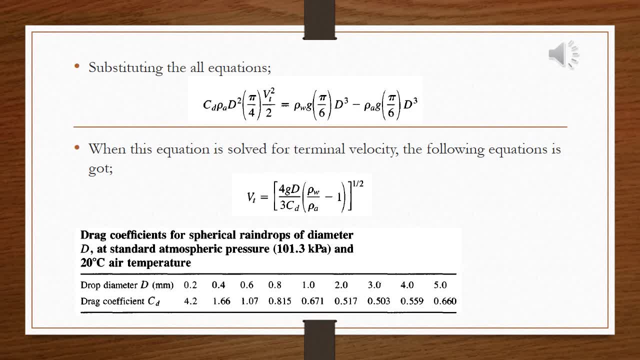 v, terminal, square over two and is equal to: here is the gravity force and minus the buoyancy force. okay, so if we take the, the in the left sides, the terminal velocity is gonna give us uh, four gravity, gravitational acceleration over the. the rain drop the diameter over three. 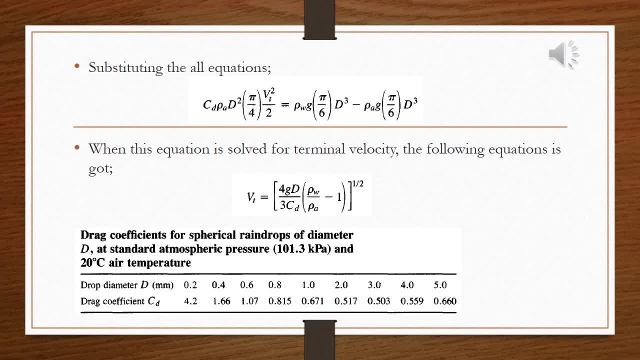 coefficient of drag multiplied by density of water over density of air, minus ones, all of them square root, given the approximate drag coefficient by diameter of drop. so in 0.2 mm of drop diameter the drag coefficient is 4.2, 0.4, 1.66 and 0.6, 1.07, and it goes on in this table all. 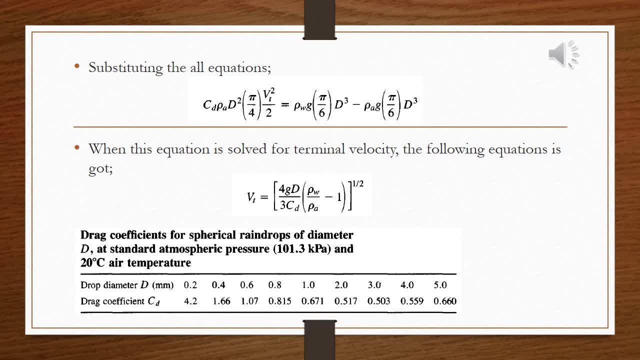 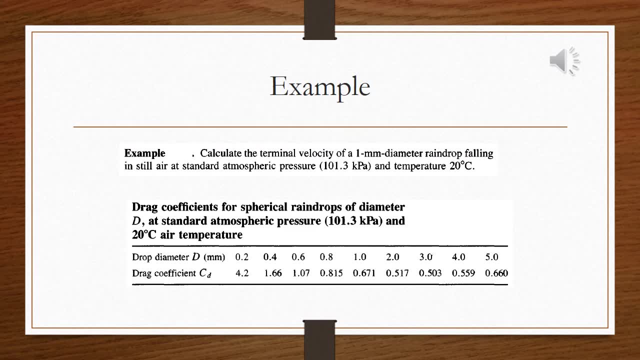 the drag coefficient at atmospheric pressure and 20 centigrade degree of air temperature. Here is an example of a thermal velocity of 1 mm diameter rain drop falling in still air at standard atmospheric pressure, which is 101.3 kPa, and temperature, 20 centigrade degree. 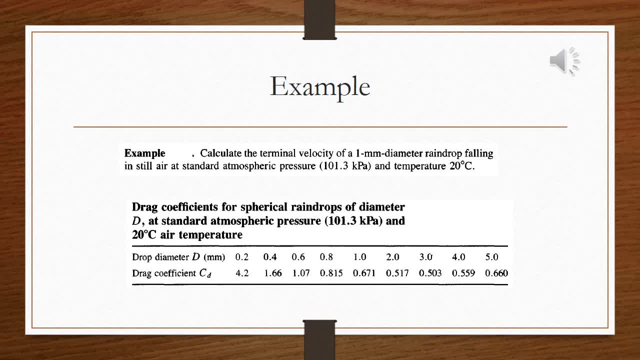 We need here for this question, the drag coefficient for 1 mm, which is in this table, is given 0.671 and we need, at this condition, which is atmospheric pressure and 20 centigrade degree, the density of water and density of air. Let's go through and then solve this question. 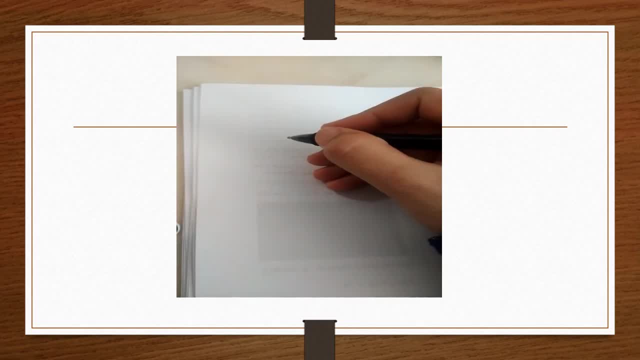 In this question we are going to find 1 mm diameter of rain drops. How many drops falling to in order to determine the terminal velocity? We know that the terminal velocity formulation is equal to four: gravitational acceleration. diameter of rain drop over three, coefficient of drag or multiply by density of water. and. 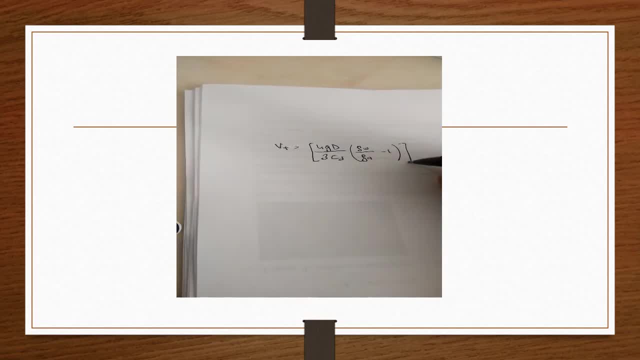 over density of air minus one, All of them's square root. We have to know at temperature, 20 degree and at 101.3 kilopascal air. At this condition, what is the density of water and what is the density of air? 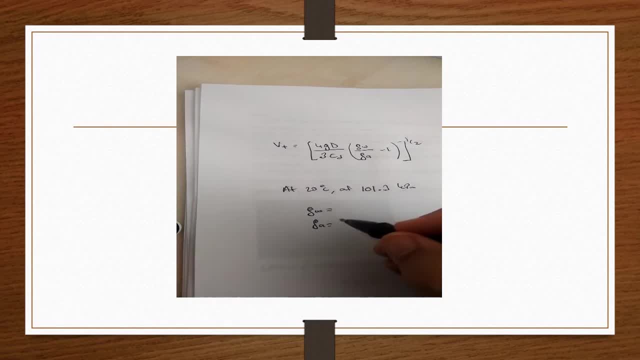 It's given- or you need to check the table- that it's going to be 998 kilogram over meter cube and density of air is around 1.2 kilogram per meter cube. at these conditions, Then we just need to calculate the terminal velocity. 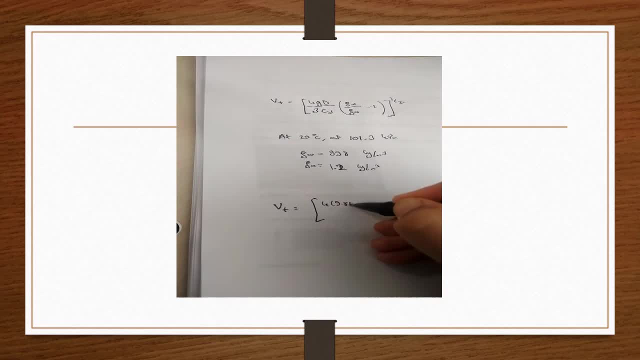 So 4 multiplied by 9.81, which is gravitational effect, It's 1 millimeter, so it's going to be 10 power minus 3 meter over 3.. And coefficient of determination we need to find from our table, which gives 0.671.. 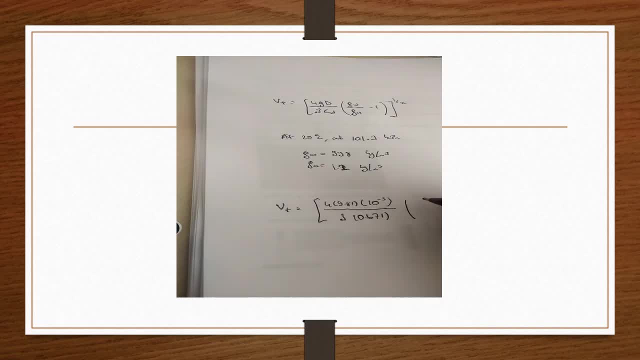 Then we need to multiply. Density of water is 998 over 3.. Density of air is 998 over 1.2.. Density of air is minus 1.. So all of them square root. Sorry, All of them square root. 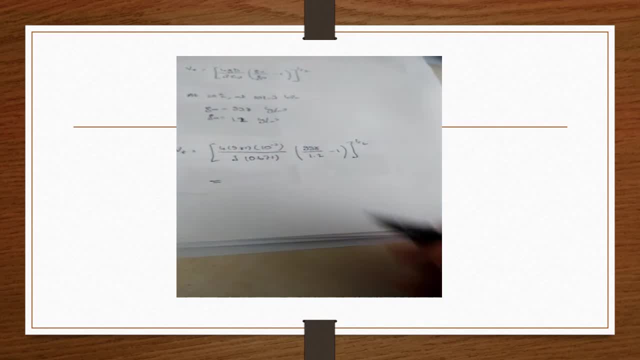 This answer Now, when we substitute all the variables and then if we calculate, it is going to give us 4.02 meter per second of terminal velocity, When the 1 millimeter, 1 millimeter raindrop falling at 20 centigrade degree and 101.3 kilopascal. 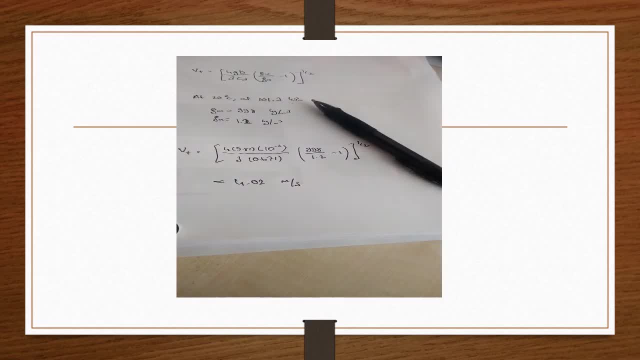 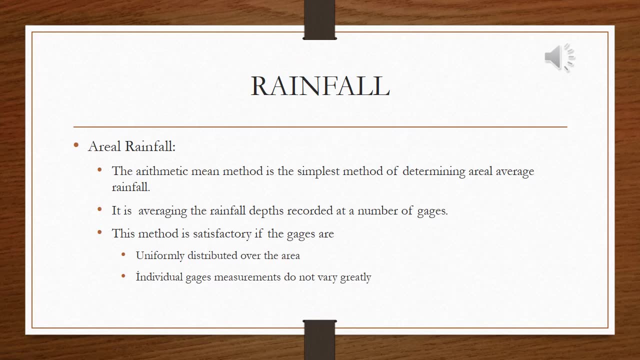 We have the 4.02 meter per second terminal velocity. Okay, Next sub chapter is rainfall. We need to calculate or determine the rainfall, How much rainfall, Amount of rainfall In one catchment. So in order to do this one, 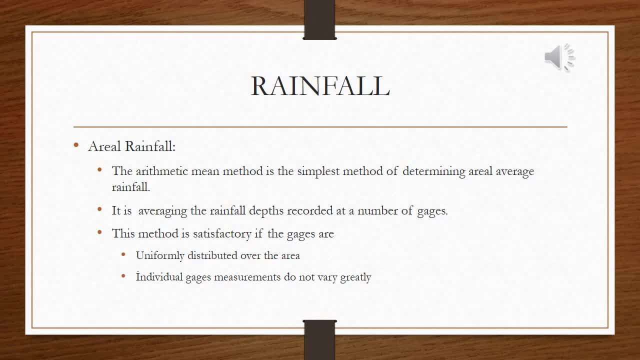 We are taking the aerial rainfall, We have couple of methods, Which is several of methods, Which is like arithmetic mean method, Theism method, Eise-Heitel method And so on. The arithmetic mean method is the simplest method Of determining aerial average rainfall. 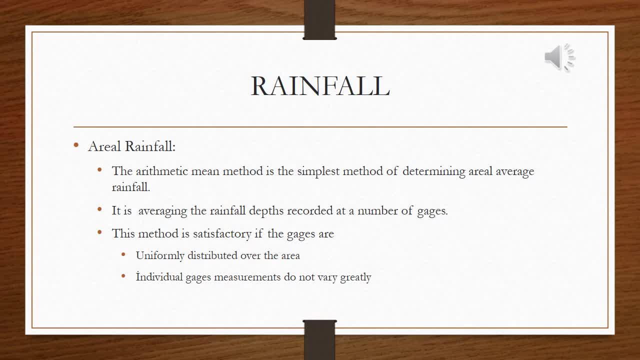 It is averaging the rainfall depths recorded at a number of gates. This method is satisfactory if the gates are uniformly distributed over the area. So the- If you take the area is going to be All of them is taking the same portion of area. 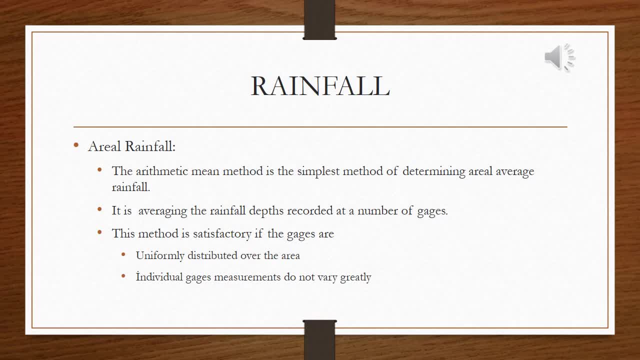 And individual gates measurements do not vary greatly, So like if one of them Is, Let's say, 5 millimeter, The other one is 50 millimeter, Is not valid This Method, So we need to apply the other methods. 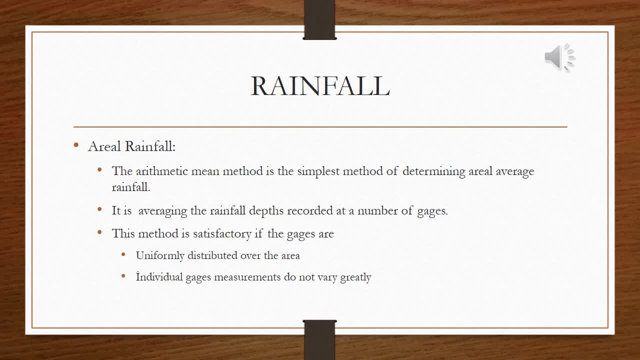 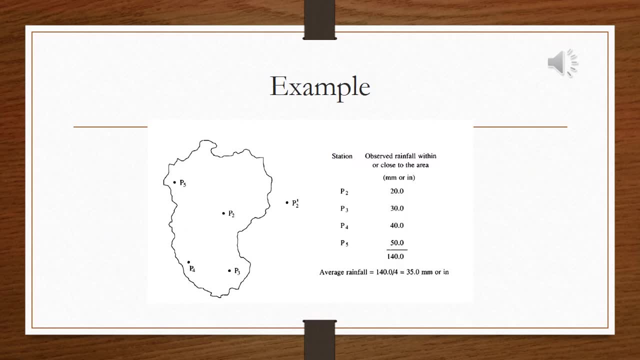 Okay, So like it's, If it is 5 millimeter, The other one is 6.. Or like 4. Or 7. Is fine, Let's see graphical representation of the arithmetic mean method. We have here Station like gates. 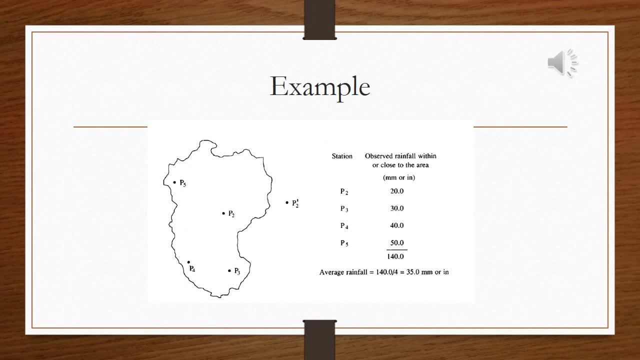 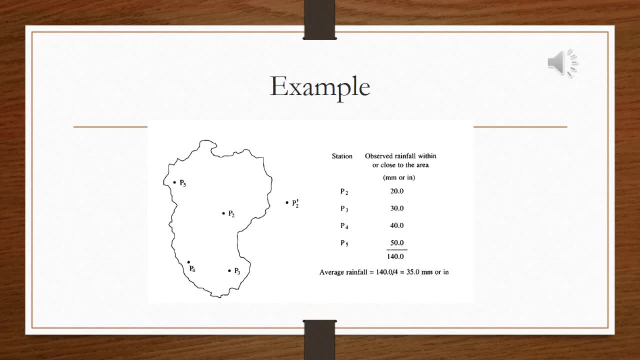 To Three, Four And Five. These are the stations. In the stations there is like a ring gates Meas, Which is measurement, And then we see that the out of the catchment area there is P2 prime. 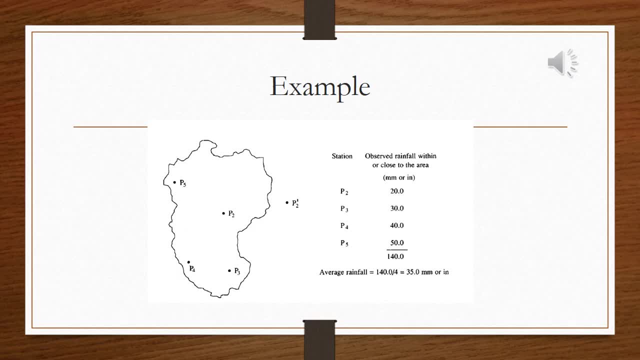 In this method, We are not taking into account this P2 prime. We just need to concentrate inside the catchment Area. Okay, So The area Is taking Over, not important, so we are gonna take only the. how much rainfall in this area? 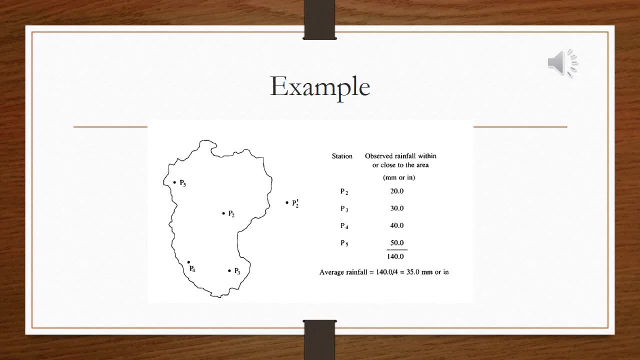 millimeter or inch. so let's see the example: in station 2 is 20 millimeters recorded. P3, which is third station, is gonna be 30, fourth station 40 and fifth station 50 millimeter of rainfall observed. we are gonna add each other. so 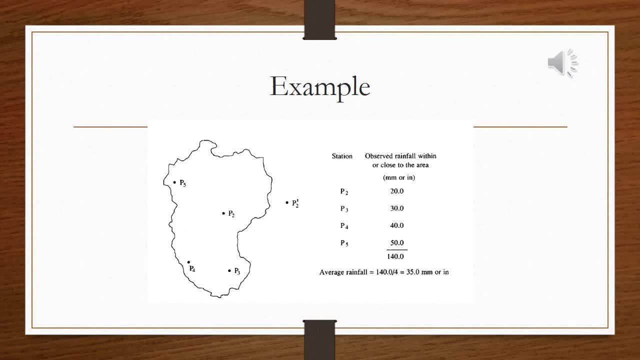 we found the total of 140 millimeters depth of height of rainfall occurred in these stations. we are gonna take the average, which we are gonna take divided 4, because we have 4 stations, so 35 millimeters of each stations, let's say. and then we are saying in this area, 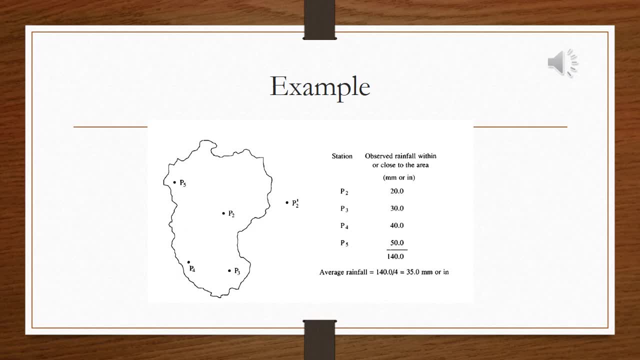 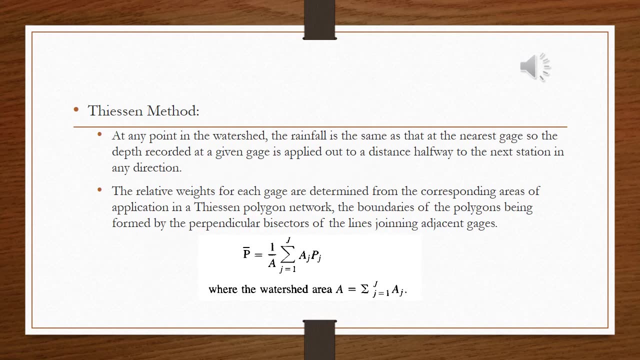 35 millimeter of rain occurred in the certain periods. the next method is the Theism method. the description of this method is: at any point in the watershed or catchment area, the rainfall is the same as that at the nearest gauge. so the depth recorded at a given gauge is applied out to a distance half way to. 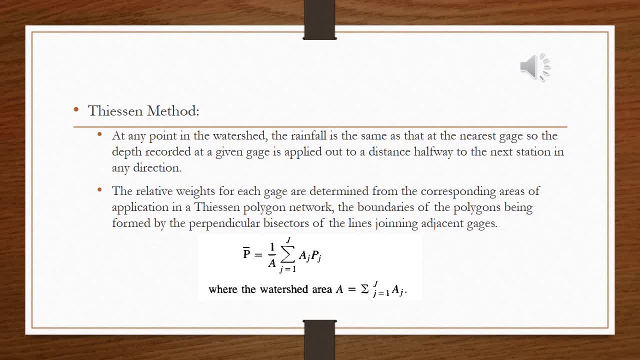 the next station any direction. so let's say we have two different stations, we are gonna draw a line and then in between we like we are, we are considering the. each station has own territory. I'm gonna show it in the graphical way in the next slide. so let's. 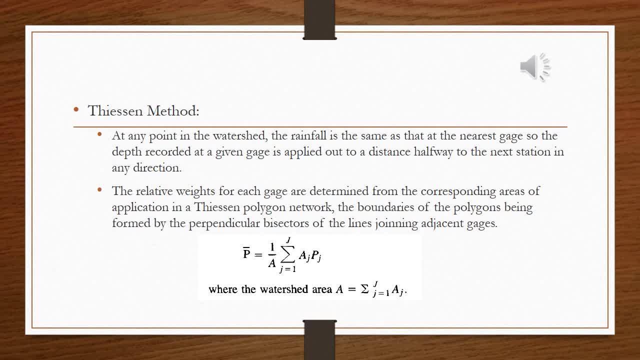 go on. the next description is the relative weights for each gauge are determined from the corresponding areas of application in a theism polygon network, the boundaries of the polygons being formed by the perpendicular bisectors of the lines joining adjacent gates. and when we do this one, let's say: 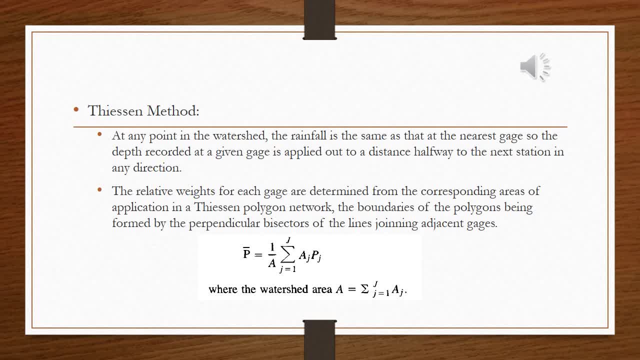 we formed our polygons and then we know all the gates inside these areas so we need to divide it totally. area of all, the multiplication of the each areas with the corresponding precipitation. so the formulation, mathematical representation, is shown here: P prime, P bar is equal to 1 over a, the total from 1 to J, the maximum number. 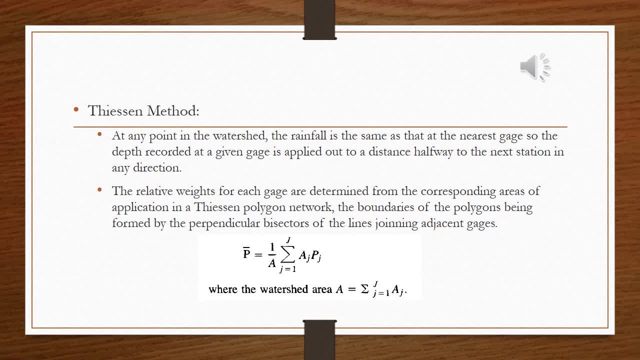 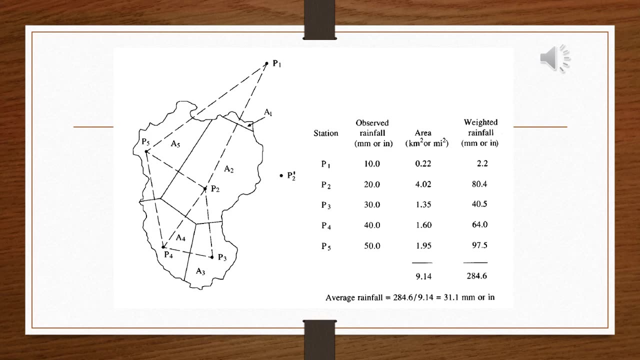 of the gates, AJ PJ, where the watershed area a is that the top, the total of the summation of the older areas. last year you guys saw how to form a ts employee polygons. if you want to remember this one, you just go back to see it. and also 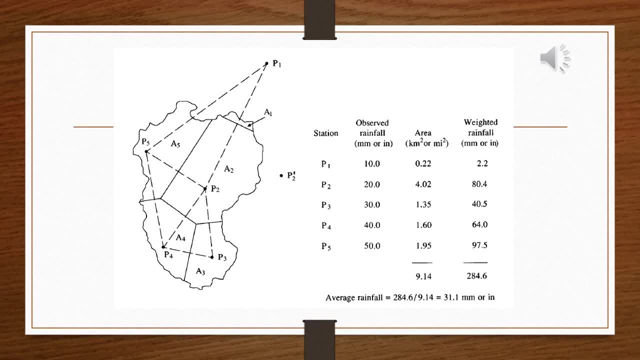 there is a computer program in order to draw a line and in order to save the type to the all these polygons. let's say we already formed all these polygons and we divided all the areas into corresponding station. and if we say less, the first station is, even though is outside of watershed, is gonna take some portion of it, which is a. 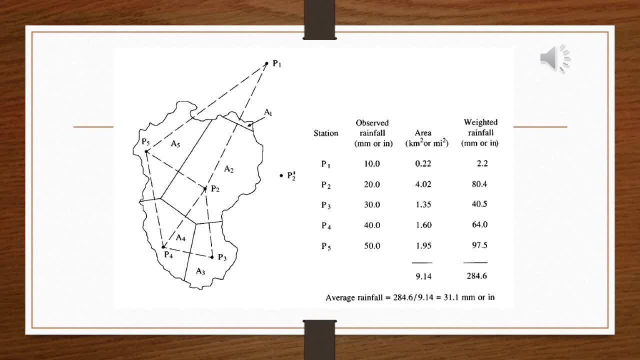 one very, very small area, but it's still applying this P one. so P one is like 10 millimeter is observed. we need to multiply by a one which is zero, point 22, very small portion of this total watershed. then P two is 20 millimeter. 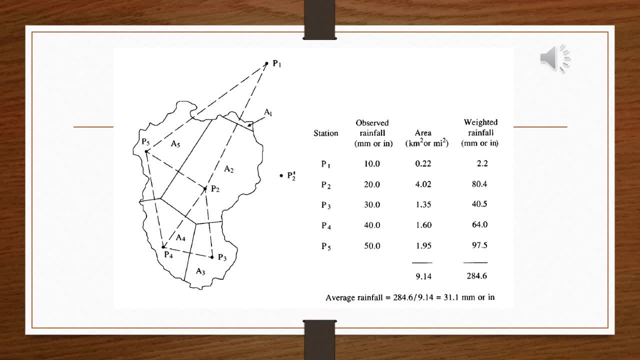 thirty, forty, fifty minute millimeters. all these stations is gonna multiply by the corresponding area and then we are gonna be find the weighted rainfall. in the last column we are gonna add each other, we are gonna find the total area is nine point fifteen, fourteen kilometer squares, let's see. and the weighted rainfall is 28 284 point six. 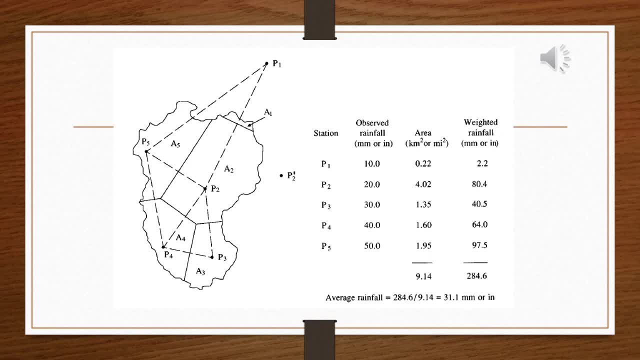 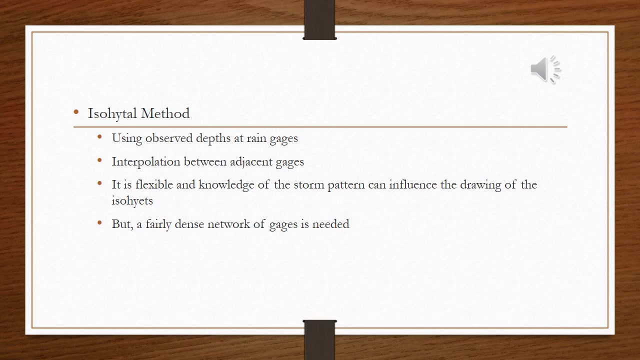 millimeters. so when we divide 200 for 284.6 over nine point fifteen is gonna be thirty one point one millimeter of rain is occurred in this watershed. another method is isohytal method. in this method use observed depth at rain gaze interpolate between: 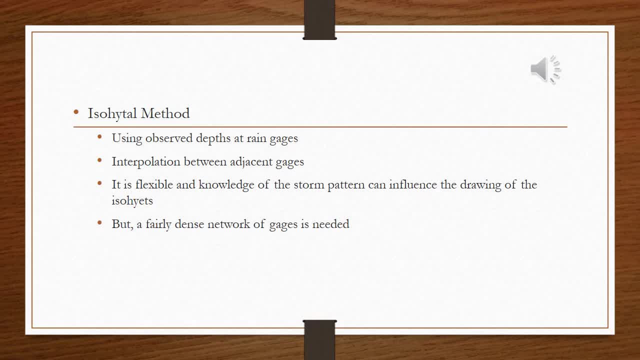 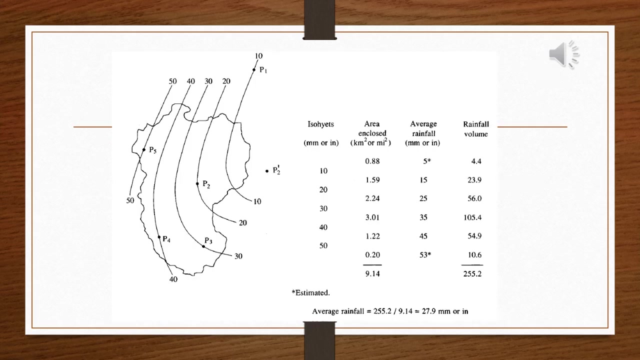 adjacent gates. Its flexible and knowledge of the stone patterns can influence the drawing of the isohites, but a fairly dense network of gates is needed. So there is an advantage and then a disadvantage of a fairly dense network of gates is needed. The graphical representation of isohytal methods as shown is showing the 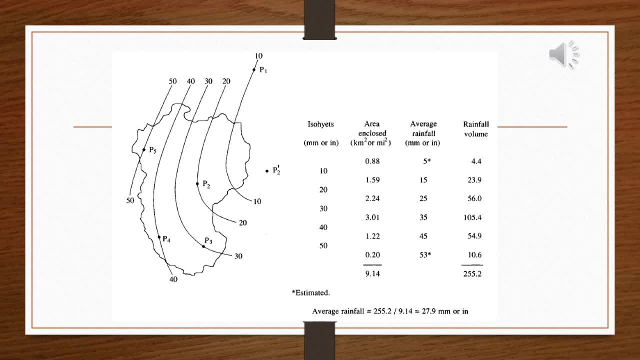 depth of the corresponding lines is like a contour map. We see here 10,, 20,, 30,, 40, 50 millimeter of depth in this, following isohites. As you see, 10, we see there is a two portion of area on the right side and 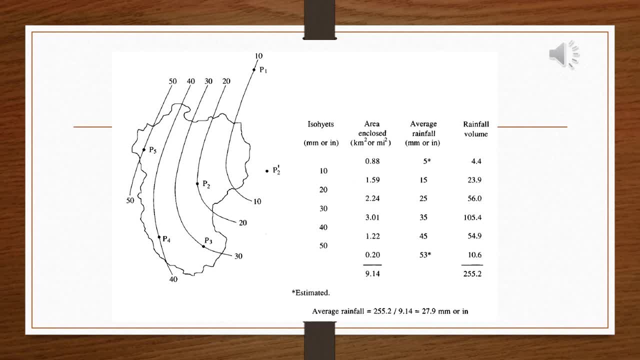 the left side. so we are gonna take, let's say, we have the 10 millimeter of rainfall occur in p1 stations, isolates and we draw a line to is 10 millimeter. 10 millimeter rain occurs in the watershed. we are going to take right side is the 0.88 millimeter kilometer square and the left side. 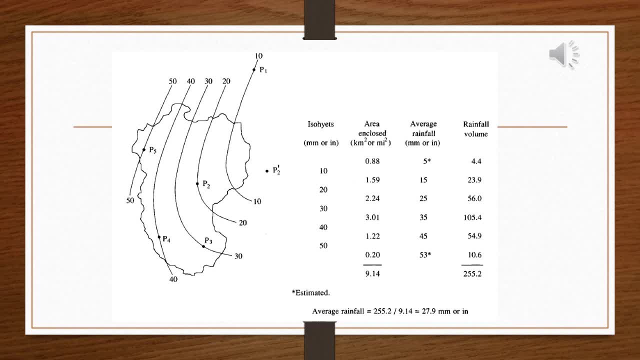 is 159, then we are going to divide it at this: 10 is 5 to 15. right, we are just gonna uh, just saying like a representative, you can make it this 5 as like 8 or something like that as well, but we are just gonna round it up. so we just need to multiply with this 0.88 area with 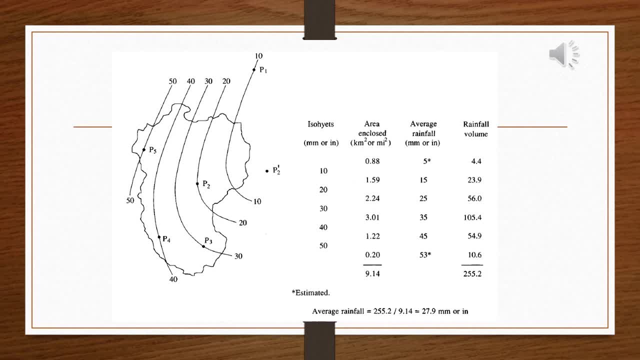 the average rainfall and we are gonna find rainfall volume. then we are gonna add all this variable, then we find 255.2 rainfall volume, total of rainfall volume in this catchment area and 9.14 is we know that is the watershed area or catchment area. so when we divide we found 27.9. 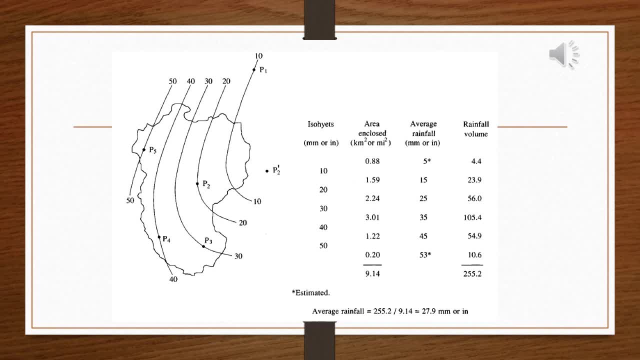 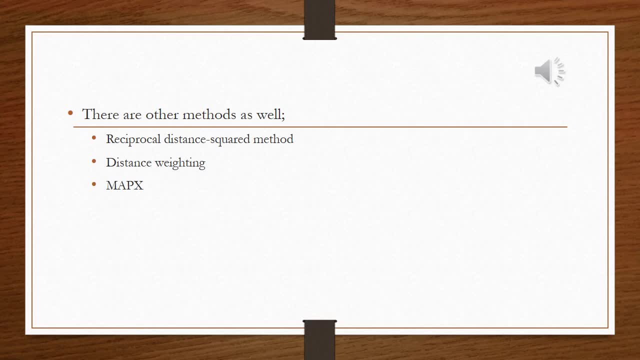 millimeters or inch of rainfall occurred in this watershed area? of course there are not. there are many other methods in order to find determined rainfall or precipitation, which are reciprocal distance squared method and distance weighting or MAPX. so this is out of our scope. I just showed you, guys, the common approach of how can you calculate this precipitation, which 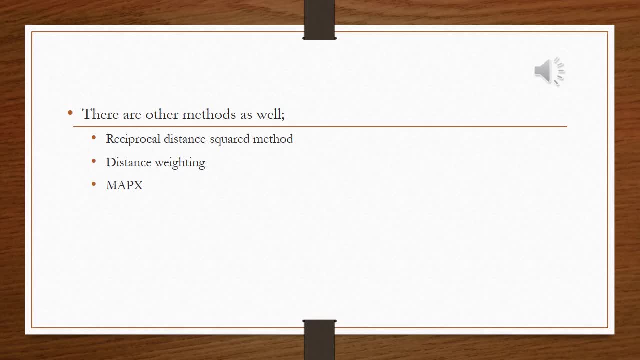 you already decided that you need to calculate distance, choosing this method. i am gonna explain, you see, in your hydrology class. uh, this is just a reminder of how we determine. and just you like, uh, when you guys see, you guys are demanding and we can go further. 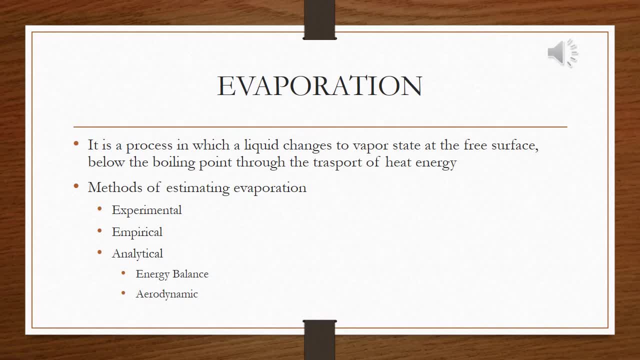 after we finish the precipitation part and then rainfall part, now we need to cover the evaporation. evaporation is a process in which a liquid changes to vapor state at the free surface below the boiling point, through the transport of heat energy. so is phase change and with the 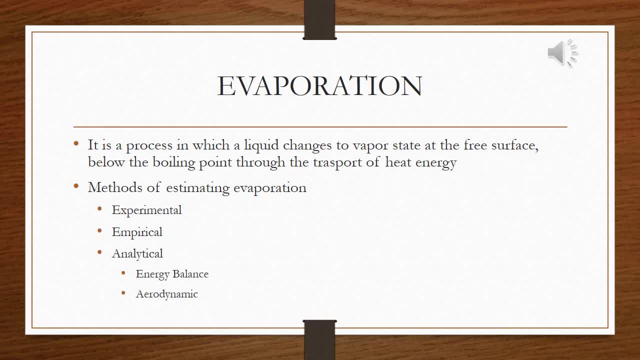 heat occurred in this process. so in civil engineering or hydrological us, we know that this liquid is water and this heat energy or heat source is sun radiation, and methods of estimating evaporation is fairly hard. but we are gonna cover uh some analytical method, but mostly it is experimental and empirical formulation. uh have in this uh area study area. but 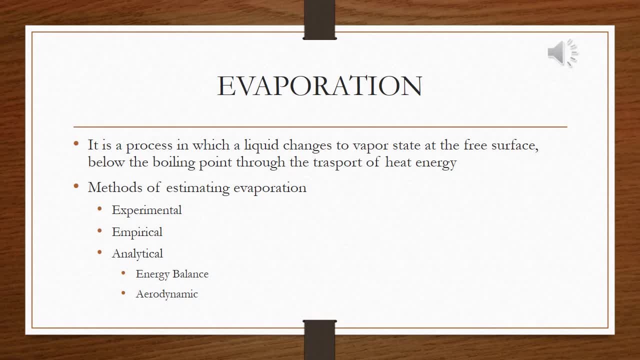 in analytical, we have two models, which are energy balance and aerodynamic method. uh, we are going to cover this analytical method because we have, um, like mathematical equation which is uh giving you like, maybe like 10 to 15 percent error margin approximately, uh, but it's uh good enough to know the analytical method. 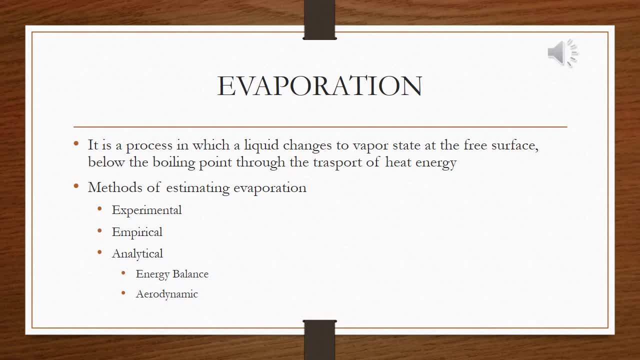 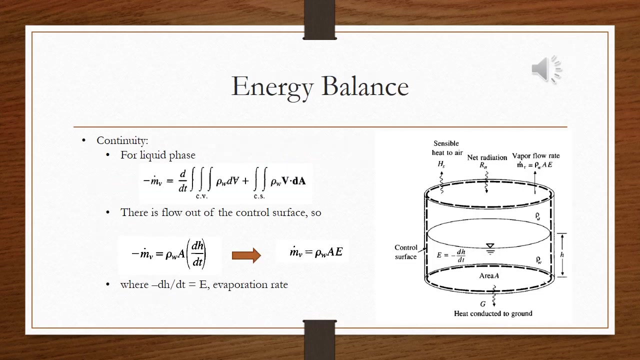 method rather than empirical, experimental, because we know that evaporation or precipitation or rainfall or whatever like, like transpiration, this is all depends on time and space, right? so that's why it's better to have the analytical method. the first is energy balance. uh, in the right side we see the graphical representation of 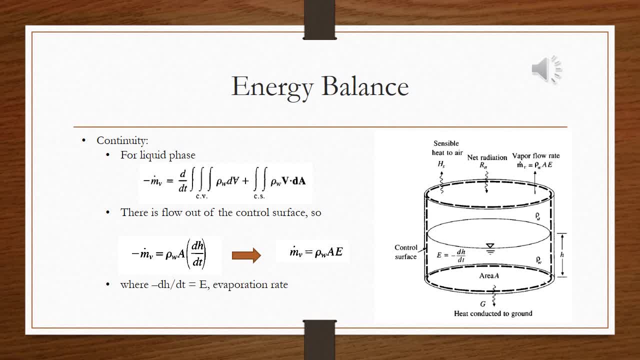 a water pan which is filled with water till the depth of the hash and it's open air, so the net radiation goes inside to heat the water inside the pan and it's evaporation because of that. it's the, the liquid water. so we, as we see here, we have heat conducted to ground, so there is an. 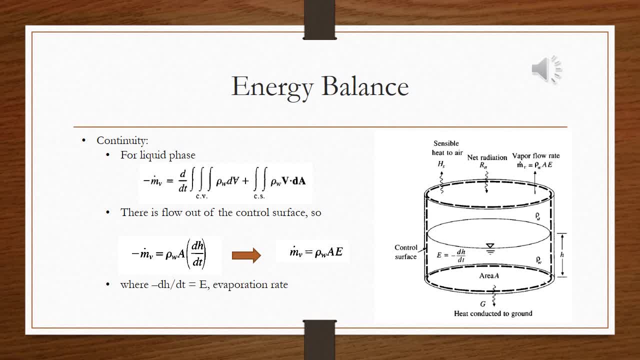 heat goes the ground, decrease the energy of this radiation rn and also the sensible heat to air. so it gives also the energy to the air as well. so we have a control surface, we have density of air and we have density of water and area. the corresponding area is. we are showing as a in order to do this. 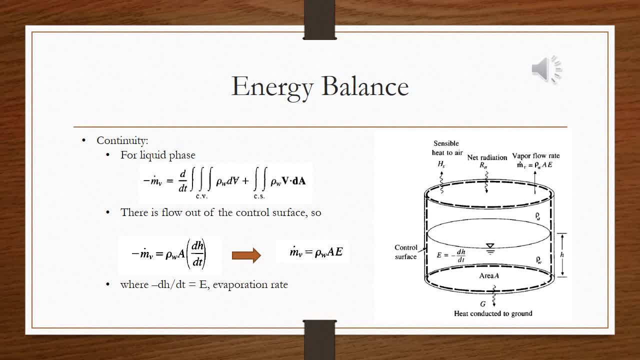 energy balance theorem. first of all, we need to make the continuity equation. we have two faces, multiple faces, which is, uh, water and air. so first let's do the liquid phase, which is water, as we know that if we want to derive the continuity equation, we take the 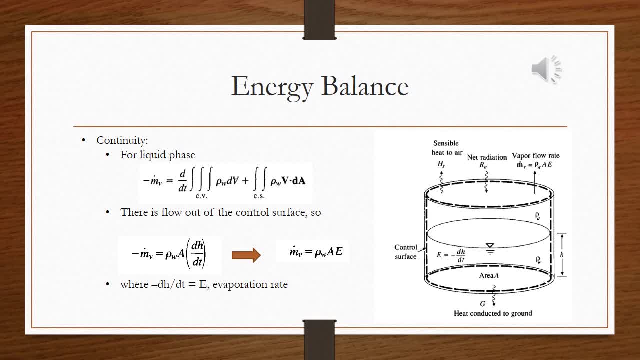 extensive and intensive properties. extensive properties is the mass, and intensive properties is dm over dm, which is one we are taking, and at the end we have minus. m, uh, mv, dot y. this is minus because we are losing water. that's why it's going to be minus and is 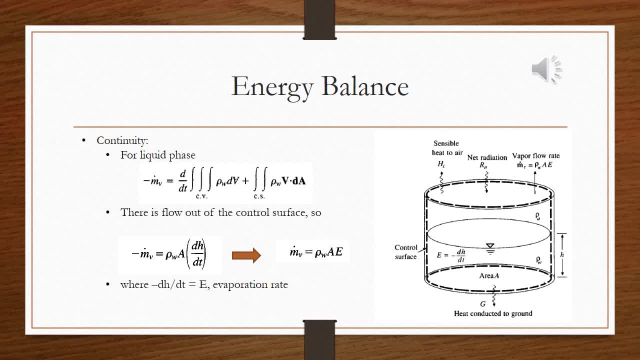 equal to d over dt. triple integral, the control volume of rho v dv plus the surface integral of rho v, b, ea. because we are taking the water, there is no income or outcome, so the velocity of this water is 0, right? so the surface integral is goes to 0 because V is 0 and 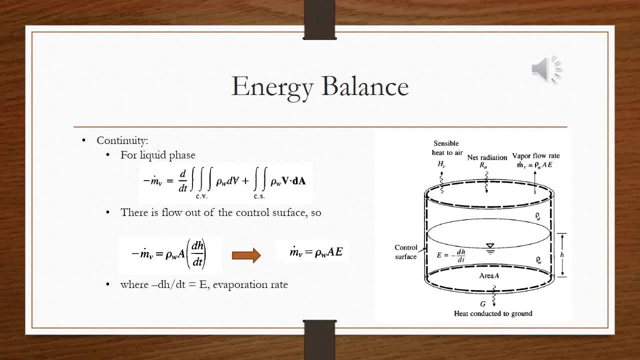 we only have the control surface of Rho V, dV and D over dt. so we know that the volume integral with the Rho V is constant, is incompressible fluid. so Rho V can be outside and area is not changing, only the height is changing. so 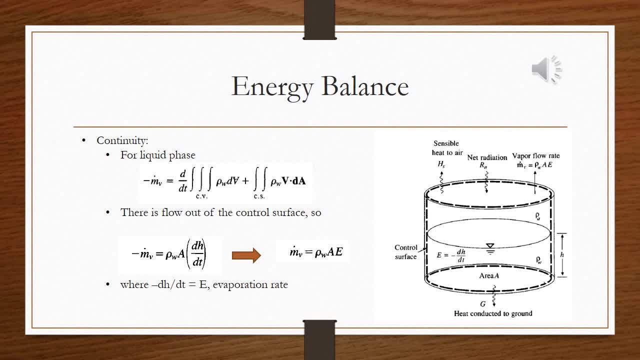 only we can take the dh over dt, which is dh. here the delta h, which is change of height over dt, is equal to the change of mass of water minus change of water. this is equal to mv. dot is equal to density of water area and e, which is this: e is dh over minus, dh over 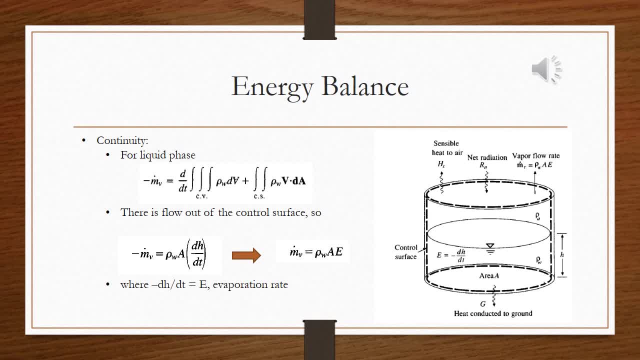 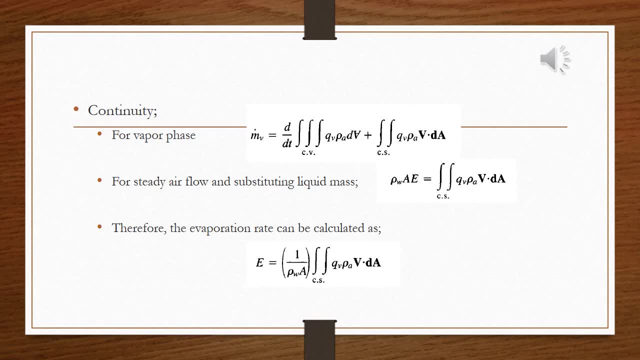 dt and it is evaporation is called evaporation rate. after we complete the liquid phase, let's go to vapor phase, because it is multi phase flow right. so the water vapor for water vapor. we wrote again our continuity equation as follows: m dot v is equal to d over dt and control volume: integral specific humidity: Rho A dV. 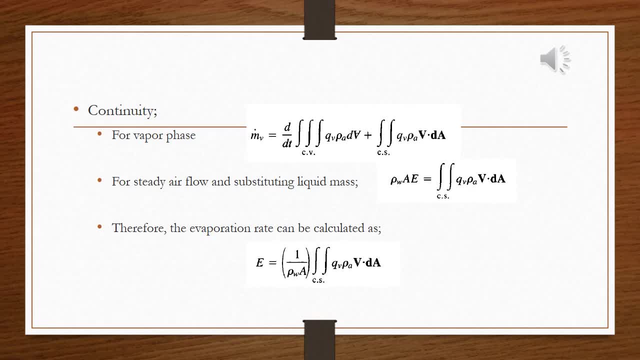 plus control surface specific humidity, Rho, A, V, dA. why it's not one? and is specific humidity? because the we said the second lecture of this class. the mass of air has different compounds rate of water and the mass of air has different components rate of water. and. 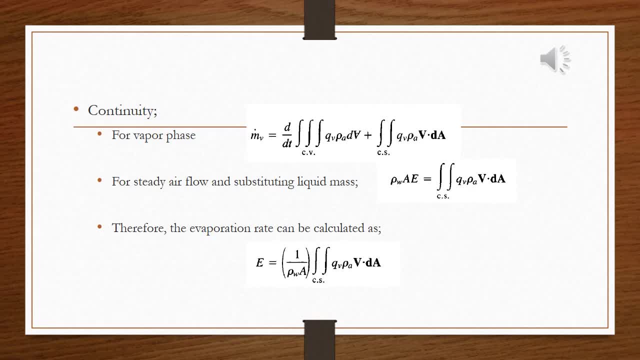 that's why we are taking the specific humidity. if you don't remember, just go back the second lecture and then you will see how we derive this equation. for steady air flow and substituting liquid mass instead of the mass of mv dot, we can say the density of waterقة and e. we have the same equation. but if we take the density of 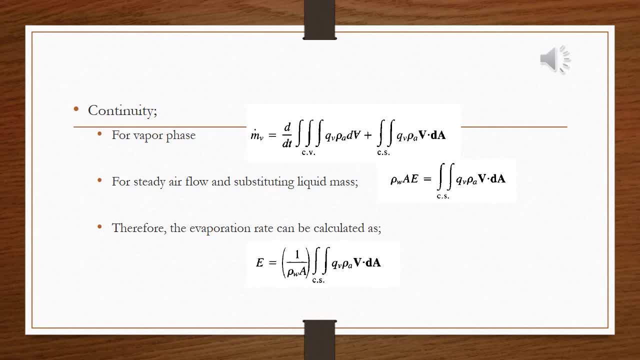 air. we can say the density of water, that's the least. the density of air and the density evaporation rate is equal to the control surface of Q, V, Rho, A, V, dA. the control volume is gone because it's steady state. so let's take, let's say it's too much. 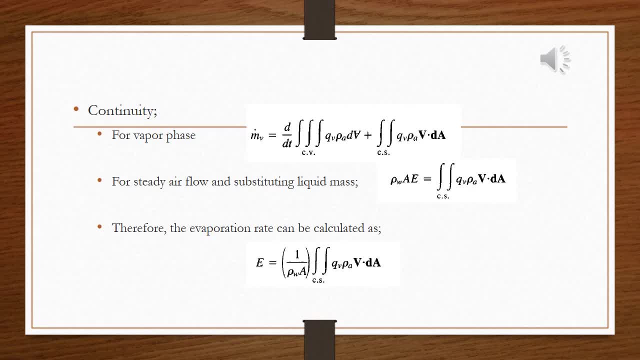 time is a long time period, and then we are taking just a steady state and it's zero and therefore the evaporation rate can be calculated here as we are taking to the evaporation rate. and then we divided Rho, VA, both sides, so it's gonna. 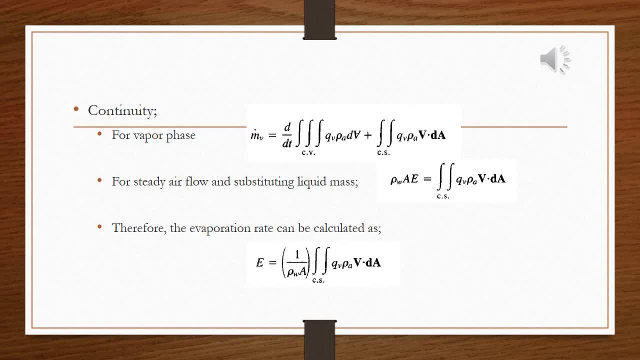 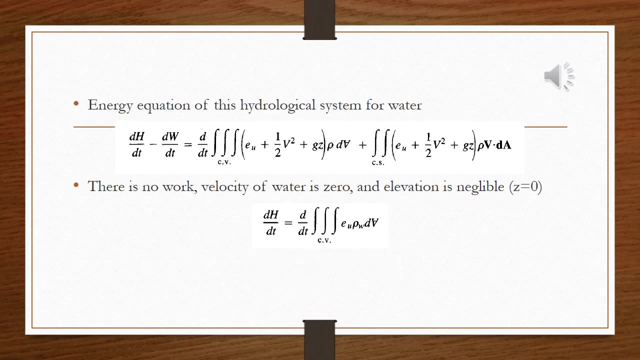 be easy- is equal to 1 over density of water area, closed parenthesis. and then we are going to take the surface integral of Q, V, Rho, A, V, dA. then we completed the, The continuity equation for both liquid and gas states. Let's go to, right now, energy equation. We know that the energy equation, the open form of energy equation, as it follows for the hydrological system, for water, 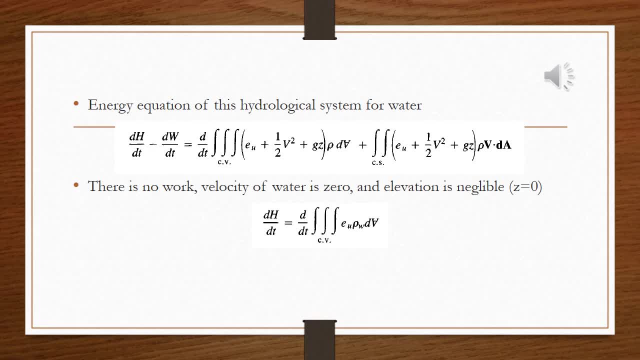 D H over D T minus D W over D T is equal to D over D T. triple integral: The internal energy plus kinetic energy plus potential energy density, multiplied by the infinitesimal volume element plus the surface integral: Again the internal energy plus kinetic energy plus potential energy density, multiplied by velocity multiplied. 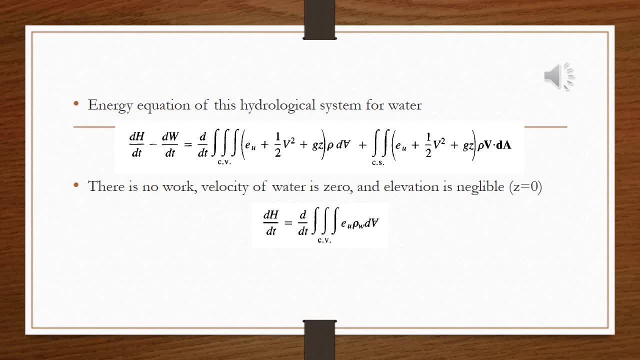 That's it. That's the product of the infinitesimal area, Unit area. So there is no work done for this system. So it's not motion, There is no motion, There's not changing anything right, It's not making any work outside the surface, or it's not taking work to make this one. And the velocity of water is zero, We know that. And elevation is negligible, which is Z is going to be zero. 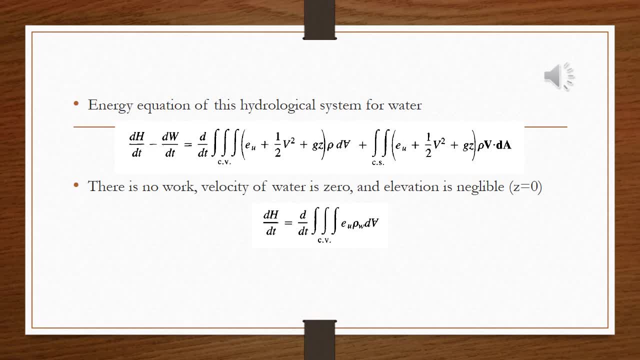 There is no change in Z. The hush in this volume is very negligible to change. So we take Z is gone. V- the kinetic energy is gone. Only thing we have here is D H over D T, because on the control surface parameter there is velocity, So it's gone. So D H over D T is equal to D over D T. 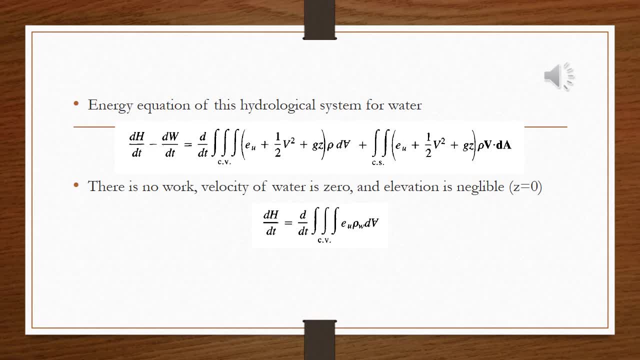 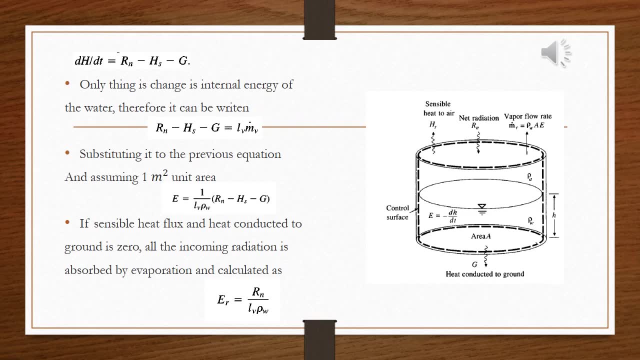 This is the volume integral of the internal energy multiplied by density of water and infinitesimal volume element As we previously depicted, the D H over D T, which is the energy. the change of energy is the net radiation goes inside this water pan, minus the sensible heat to air and minus heat conductivity. 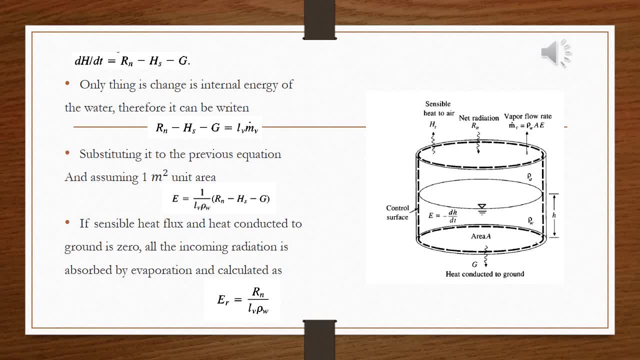 It is conducted to the ground. So it is in this balance of energy. So only thing is change is internal energy of the water. Therefore it can be written: the R N, which is net radiation, minus H, S, which is sensible heat to air, minus G, which is also the heat conducted to ground right, is equal to D H over D T. 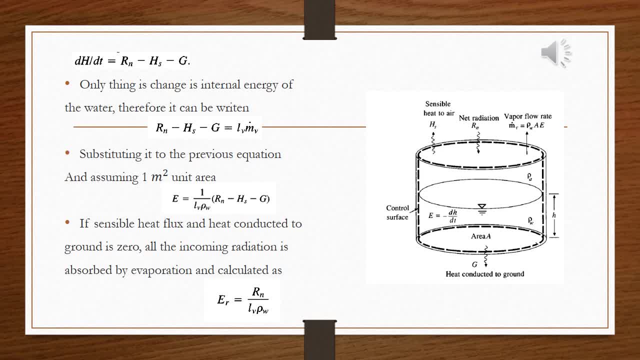 So it's gone. So we take Z is gone, So we take D H over D T, which is the energy. the change of energy is the net radiation goes inside this water pan, minus the sensible heat, As we previously depicted, the D H over D T, which is the energy. the change of energy is the net radiation goes inside this water pan, minus the sensible heat to air, minus G, which is also the heat conducted to ground right, is equal to D H over D T. 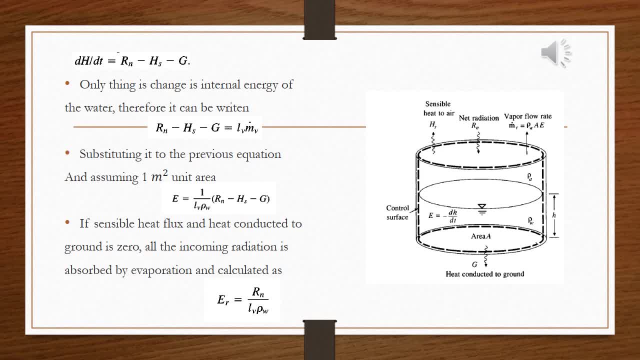 heat conducted to ground is zero. all the incoming radiation is absolute, absorbed by evaporation and calculated as er is equal to rn over lb roving. so which means if we insulated the bottom, so there is no heat conducted to the ground and let's say the air, uh, also like 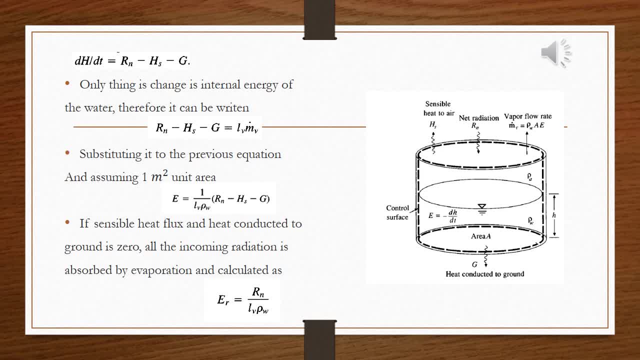 we, we avoid the lose the heat to the air, so we keep all the heat inside and we can ignore the hashes- goes to zero, so the all radiation absorbed by the water in order to evaporate this water. it's better to solve an example here in order to understand everything. 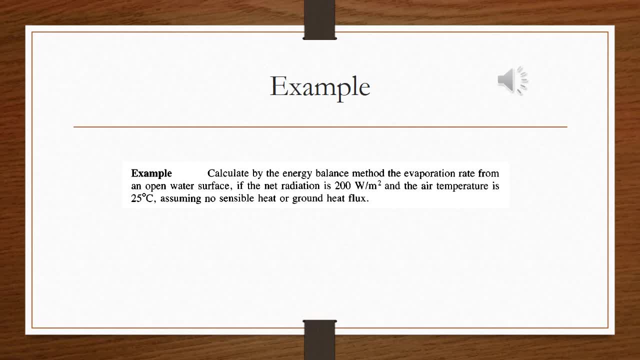 this energy balance theory. we are going to calculate by the energy balance method the evaporation rate from an open water surface. if the net radiation is 200 watt per meter square and the air temperature is 25 centigrade degree, we are going to assume no sensible heat or ground heat flux. so that means there is no h, h, s and g. 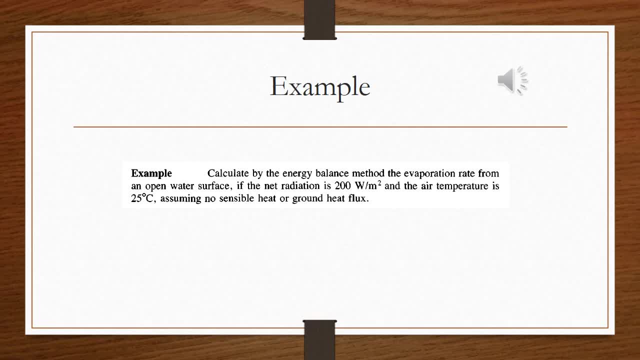 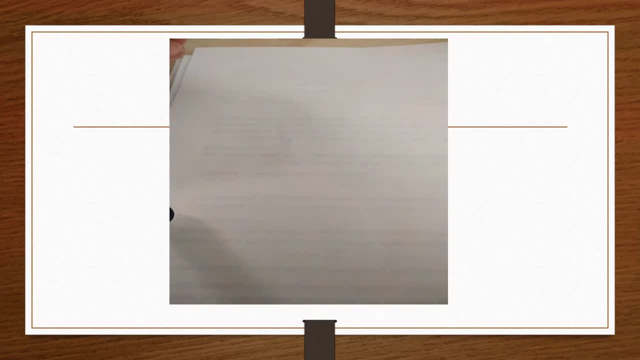 we are going to take these parameters zero, okay, in this question. uh, if it's clear that there is no ground flux and there is no sensible heat of flux into the air, so we just have. er is equal to rn, which is the radiation energy over the latent heat and the density of water. so the rn is given 200, right, is going to give us 200 watt. 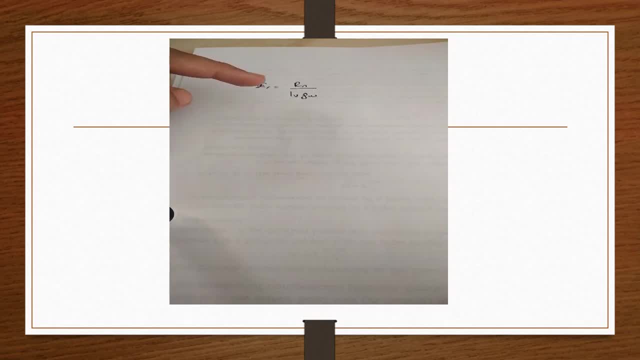 over meter square. we need to know the density of water at 25 centigrade degree, which is- let's see, rho w is, is um, let me check: is 997, 997 kilogram over meter cube? okay, and the the latent heat for 25 centigrade degree we need to have from our second chapter. i already provide that. 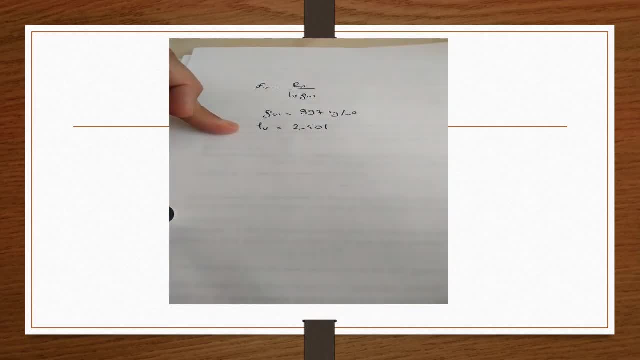 is. we have this formula: 2, 2.501 multiply by 10 to power, 6 minus 2370 multiply by temperature. our temperatures here is centigrade degree, so we need to multiply by 25 here. so it's going to be 2.501 multiply 10 to 6 minus. 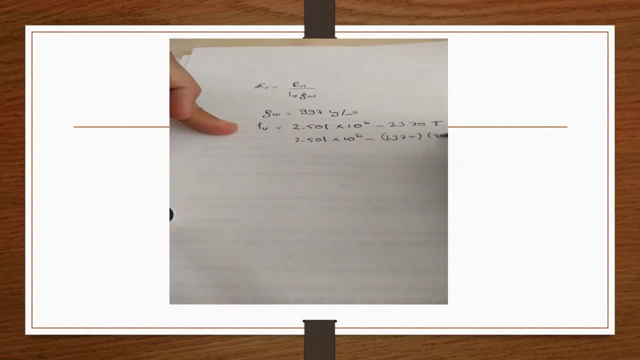 2.501, 2370, multiply by 25 um, so the latent energy is given here 2441 kilojoule over kilogram. if we take this one is going to be joule over kilogram. so i divided everywhere 1000, so in order to have kilojoule over. 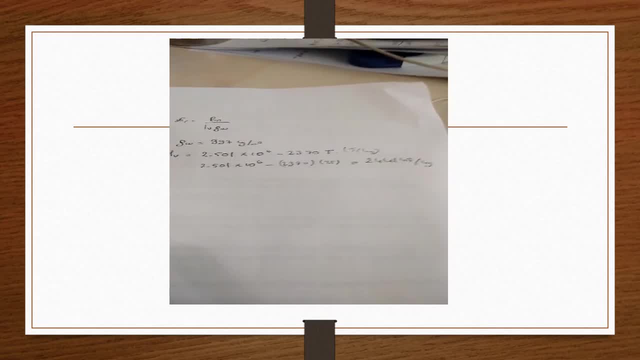 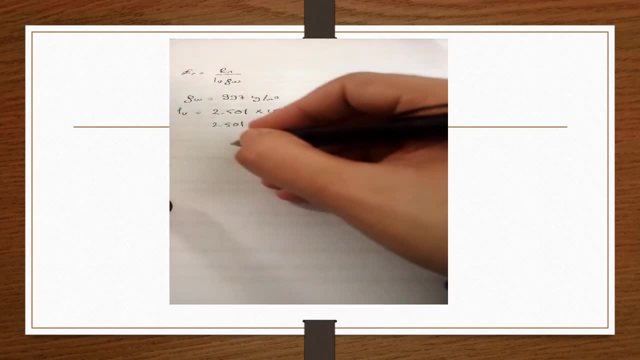 so i divided everywhere 1000. so in order to have kilojoule over kilogram, so we need to have kilojoule over kilogram, so it's going to be 312 kilogram. let me show like this: so it's going to be better soon. okay, all right, so it's just. uh, we just need to uh plug all the. 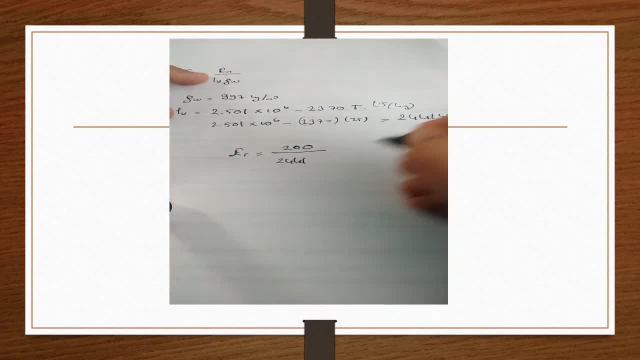 variables: rn is 200, uh warmth so it's 2. 441 is plausible, so it needed to confrontation. convert it to the Joule because this is what. so 10 to power 3 and multiply by density is 997. program over meter cube. so our energy when we multiply all this, 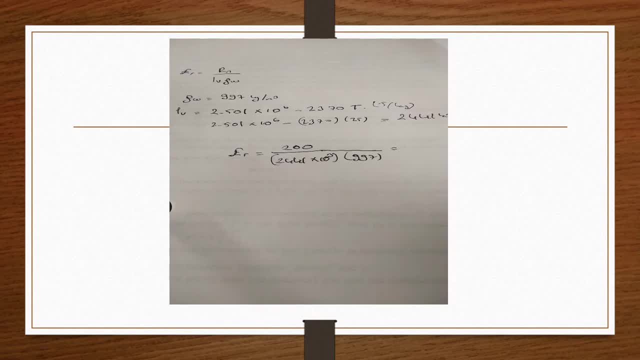 one. we are gonna have eight point. let's see here: eight point twenty two multiplied 10 to minus eight meter per second. so I'll calculate the operation rate. okay, our evaporation rate is: is eight point twenty two multiplied 10 to minus eight meter per second every. 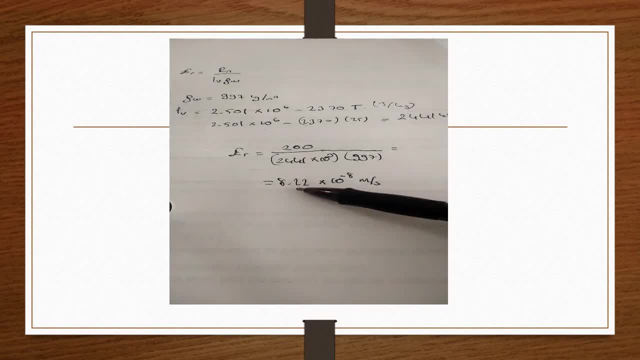 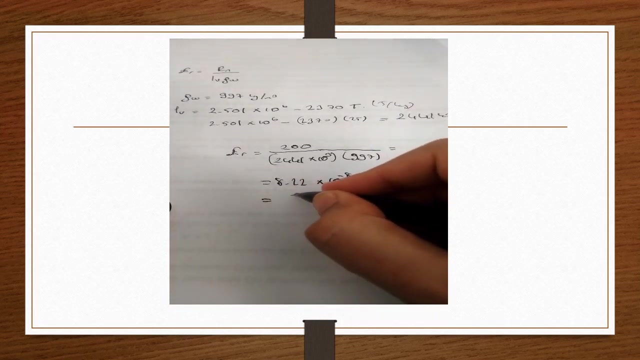 second, there is eight point twenty two multiplied ten to eight meters of water is evaporated in certain area, like unit area, okay, one meter square or something like that, if we take this one to do as what we are measuring as rain millimeters per day. so it's gonna be, if you convert, all the necessary units is gonna be seven. 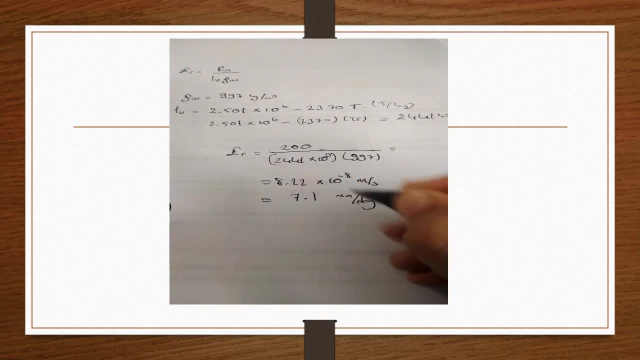 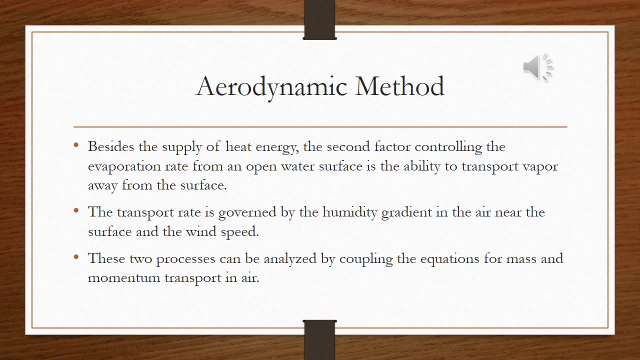 point one millimeter per day. every day, seven point one millimeter of water height is evaporated in this catchment area. the next one is aerodynamic method in for this operation, determining their operation rate. oh, In analytical method, besides the supply of heat energy, the second factor controlling the evaporation rate from an open water surface is the ability to transport water vapor away from the surface. 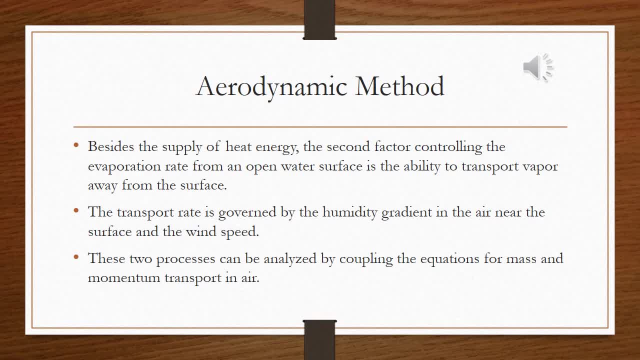 The transport rate is governed by the humidity gradient in the air near the surface and the wind speed. These two processes can be analyzed by coupling the equations for mass and momentum transport in air. So, in order to go through the details of this method, I am just going to give the important equations so we can jump to the conclusion. 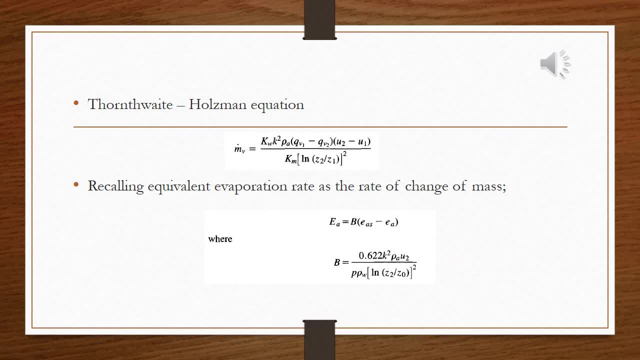 Interested reader can go through and study the details of the aerodynamic method, but at the end we are going to find this Tong-White-Hausman equation, which is the rate of change of mass, is equal to a bunch of these variables. 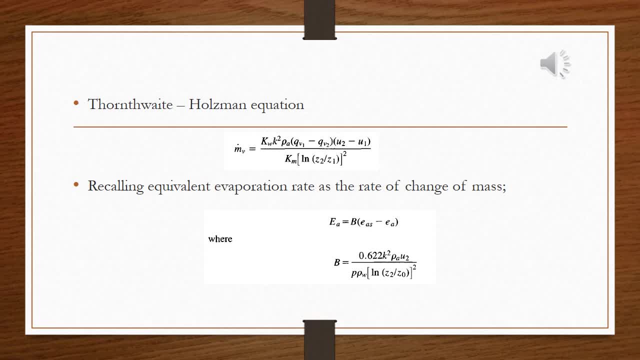 And we recall the equivalent evaporation rate as the rate of change of mass, as we do before. the rate of change, which is m dot v, is equal to, like the water mass, the density of mass and the evaporation rate, and multiply by area. 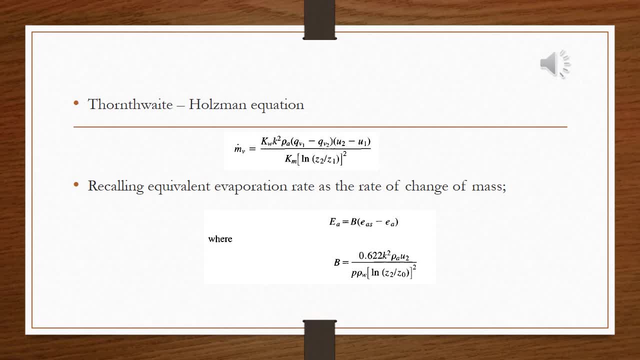 So we say the final equation is: the evaporation rate is equal to b multiplied by The saturated water vapor minus water vapor. where is b? is depends on the von Karman constant, which is k. is generally taken 0.4, square 0.4, k is 0.4, and the density of air, the velocity and pressure, density of water, and then the elevation. 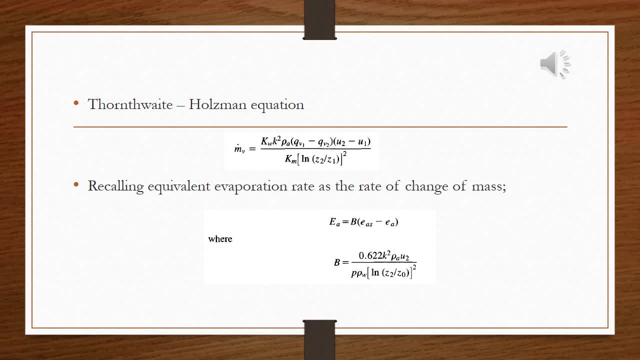 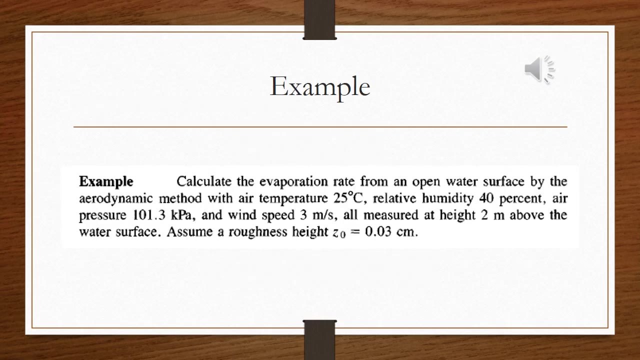 So when we use these parameters, we are finding the Evaporation rate with aerodynamic methods. let's see an example. is going to be understanding that? Okay, we are going to calculate the evaporation rate with using aerodynamic method again. is the air temperature is 25 centigrade degree and the relative humidity is given here for 40 percent. 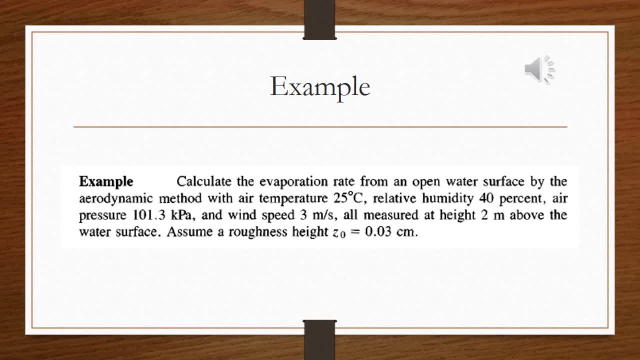 Air pressure is 101.3 kilopascal and wind speed is three meters per second, all measured at height two meters above the water surface. so we are assuming the roughness of height Z zero as 0.03 centimeter. let's see the calculation how. 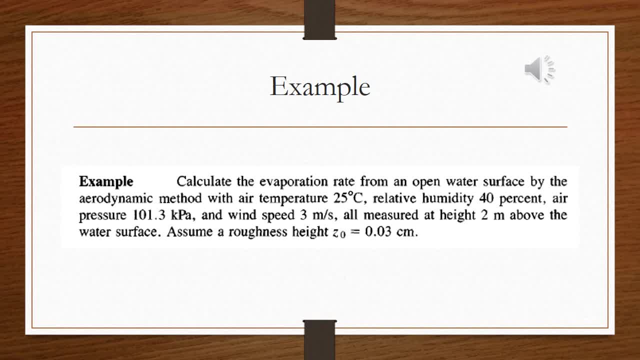 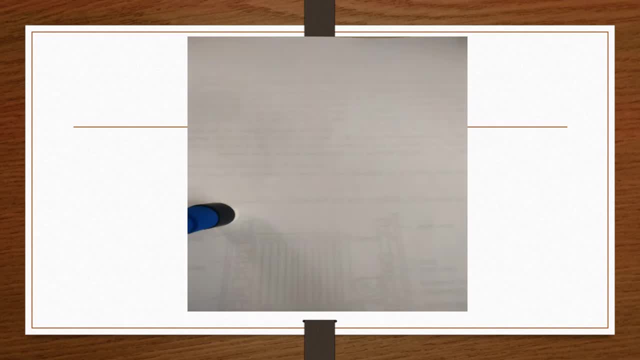 we are gonna calculate the evaporation rate with using aerodynamic method. okay, now we are gonna find evaporation rate by using aerodynamic method. in order to find this one, we know that evaporation rate with using aerodynamic method is B, which is vapor transfer coefficient, EAS minus EA. right, so water. 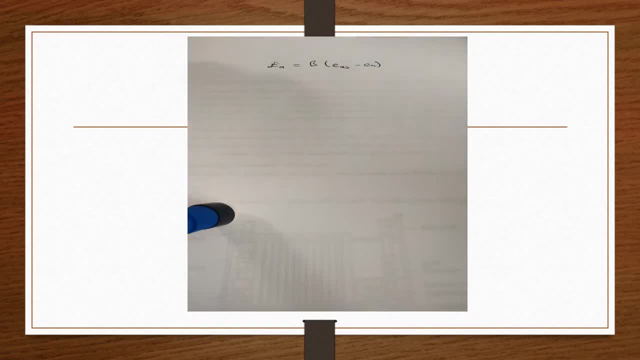 vapor saturated with water vapor minus water vapor. let's go through first today's to define B, which is vapor transfer coefficient. we know that B is equal to zero point six, two. two von karmann constant square multiplied by the wind velocity over pressure of air, water density at certain temperature, whatever. 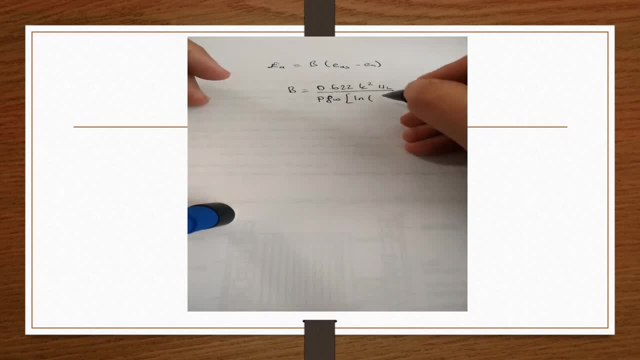 is given, and natural logarithmic of z2, which is the elevation measurement taken, and Z 0, which is the surface height, the roughness. so we can take 0 if it's not given and if it's given the roughness, we are gonna take whatever it is. if we take 0, we know that. 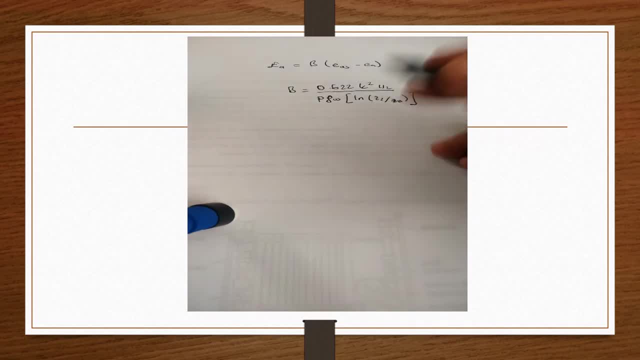 we, if we divide is gonna be the infinity. so our question is gone. so there's why we are taking a roughness, we are not taking zero, okay. okay, this B is equal to 0.6 to 2 x 0.4, which is one carman's constant square. we know that wind is 3 meter per second. 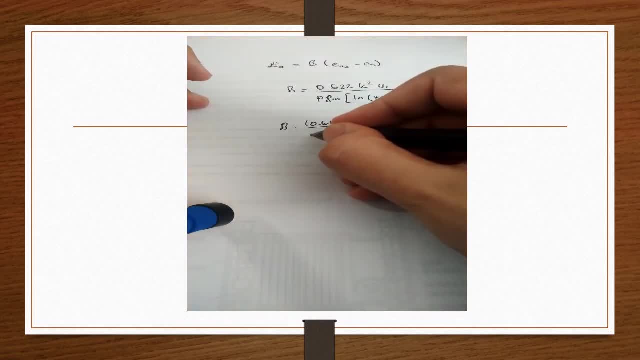 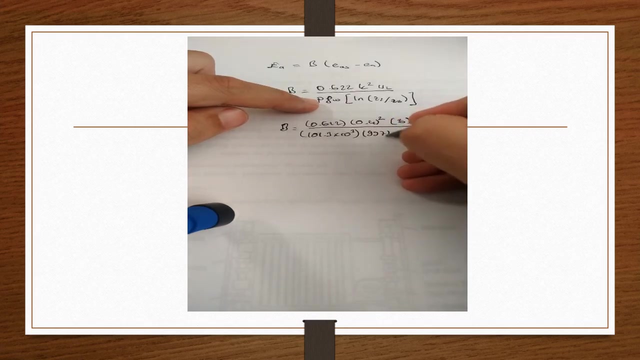 over pressure is given one hundred one point three, one under one point three, multiplied by 10: 3, it was kilo Pascal, so I turned it, converted to Pascal it. we know that the density of water at 25 degree per in the previous example is 997�-m³ to grams. micro cupes right. so 7page Y. 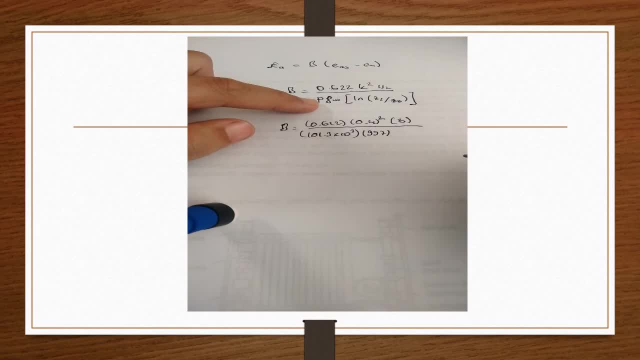 b, the same is equal to alpha, B is equal to 90.8. vorstellen more talk we find in 8.unciy A wage. we take here 556DT. the energy of transport. Cybra area is 100 lot steak 1992 us per ada state five적 competitions. so as an example, & down side Akhada state. but our 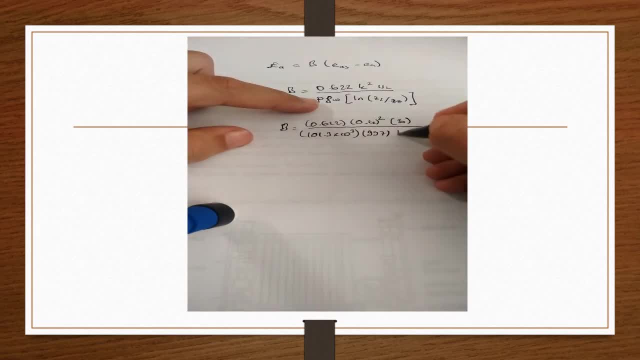 recording. we've got to Gyro and skip the, the same�ovic H1C 1967. you've got a men's, a man's meter cube and natural logarithm of z2 is 2 meters over z0, which is this: roughness is 0.03 centimeters, so 0.03- let's say in the parenthesis, 0.03 times. 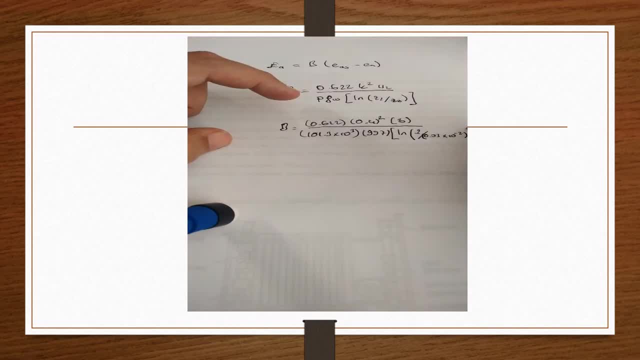 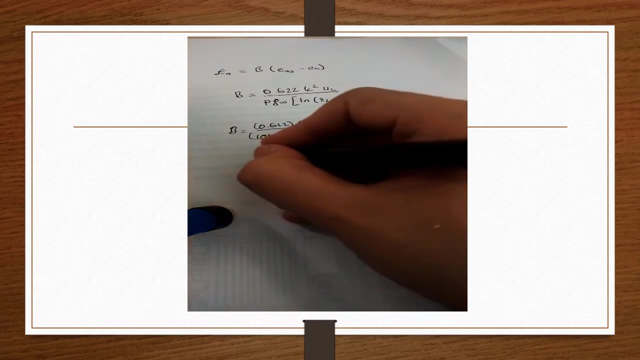 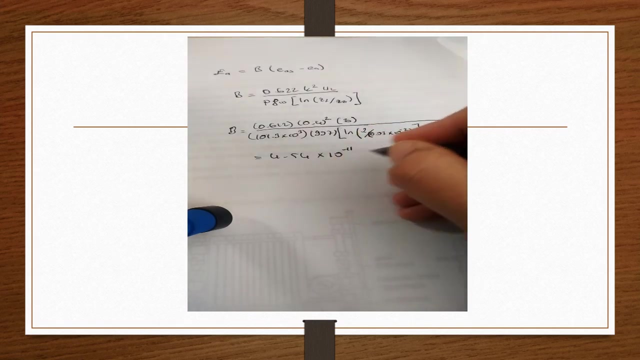 10 to minus 3 is gonna give us meters. okay, this one okay. when we plug all the variables and then when we calculate, it is gonna give us four, point fifty four times 10 to minus 11 meter per Pascal. second is our. meter per Pascal, second is our. 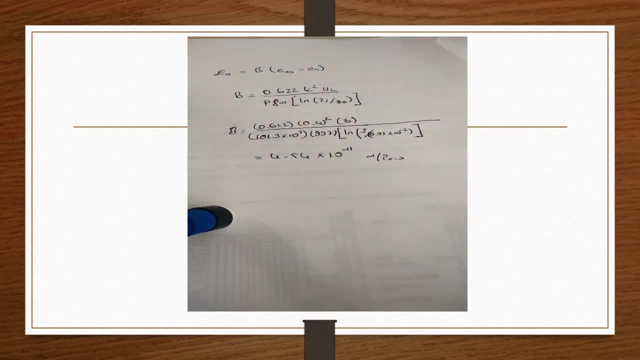 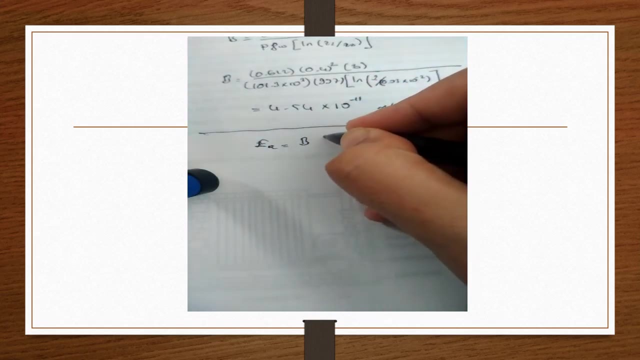 vapor transfer coefficient, which is B. okay, then, what we need to calculate. we are gonna calculate the evaporation rate, which is B. what we calculated and EAS minus EA, saturated water vapor minus water vapor at 25 centigrade degree and 15 centigrade degree and. 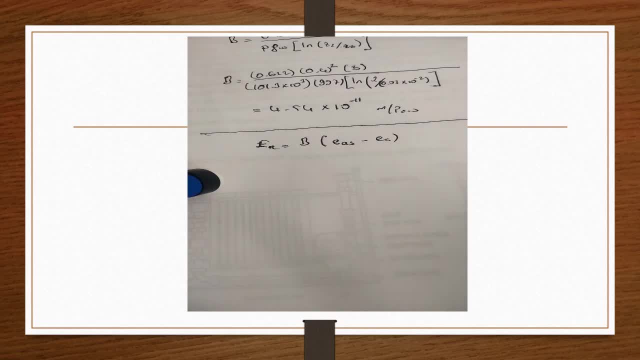 101.3 kilopascal. we need to look at the table and in this table is gonna given so at the book: 454 times 10 to minus 11, which is B, and then E, saturated water vapor minus water vapor. Water vapor is given at 25 centigrade degree: 3167 pascal. 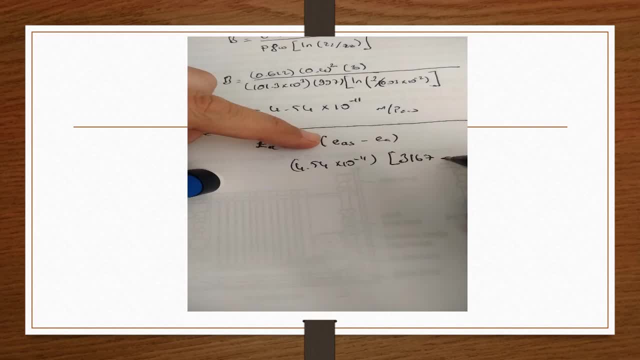 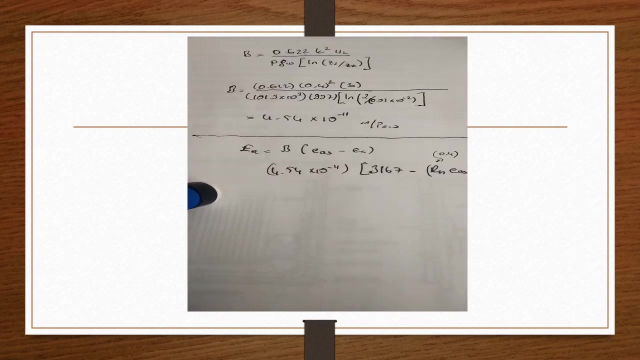 Minus. so we are going to find the water vapor, which is the relative humidity multiplied by saturated water vapor. Relative humidity is 40%, we know. So we are going to, Instead of relative humidity, we are going to- Right, let me put this one. So it's going to be 3167 minus relative humidity multiplied by the saturated water vapor. 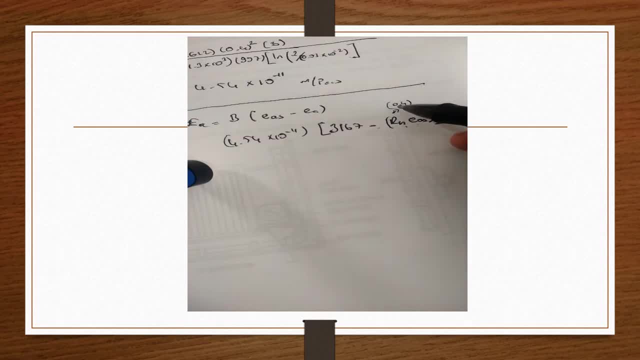 So we know that relative humidity in the question is 40%, so it's 0.4, And EAS, which is saturated water vapor, Which already we are writing 3167, 3167, So it's 0.6. So our equation is going to be: 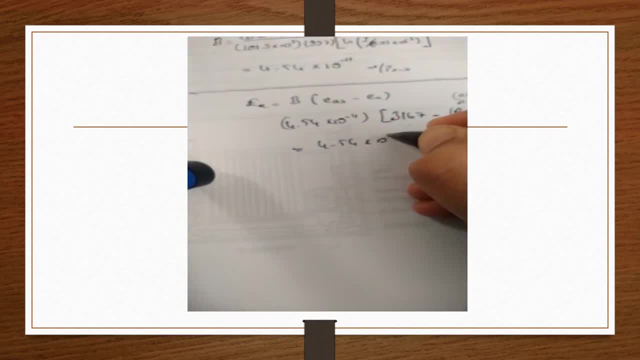 4.54 times 10 to minus 11- This is 1,, this is 0.4- Is going to be 0.6. 0.6 Multiplied 3167 Of E, saturated water vapor, So EA, which is Aerodynamic Method. 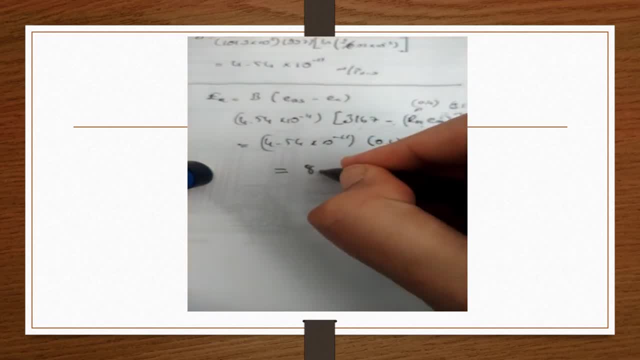 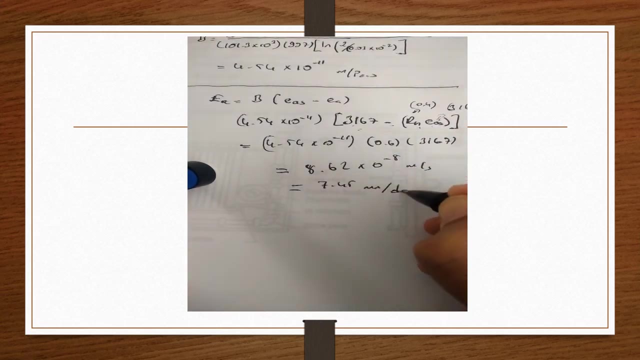 Evaporation rate is Found: 8.62 Times 10 to minus 8 meter per second. We are calculating again For millimeter per day Is going to be 7.45 Millimeter per day, So it means every day 7.45 Millimeter. 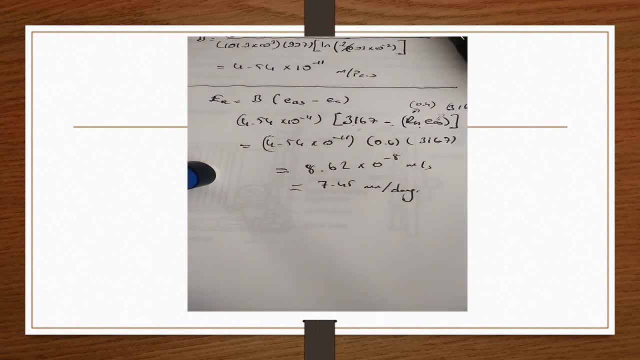 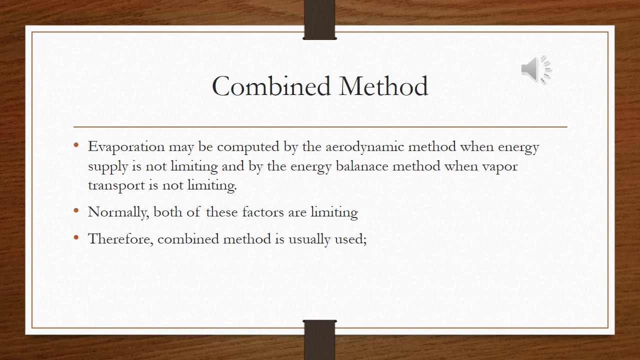 Water Is Losing Or like Liquid water is losing Vapor. In this condition, If you pay attention In energy balance Method, We see that If there is like heat Radiation From sun, Sun radiation occurs, We can calculate, We can apply the Energy balance And aerodynamic method. If we Consider the winds, 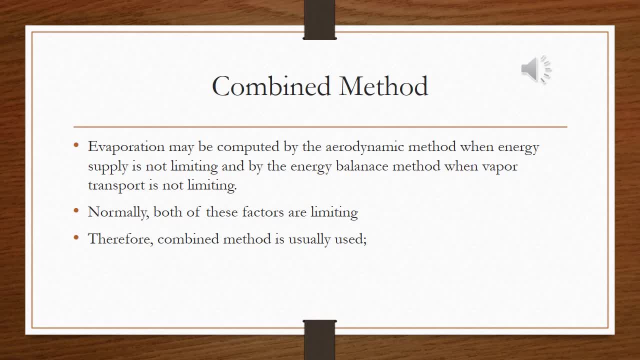 Energy and Wind speed And This the elevation And all the Constant, if we know We can use this aerodynamic Method. Let's say, If these two Are limited, Is very hard to find The sun's radiation at the current Space and time, Space and time and also The wind. 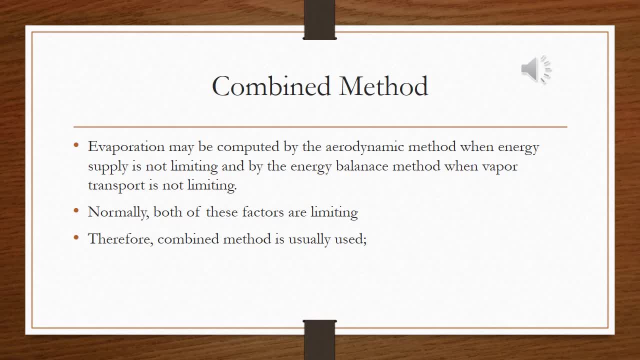 Velocity speed. We need to take into account Blah blah, So let's say it's limited. Normally both of them Are limited, right? So therefore they Develop or improve Combined method. So Combined method Is very common to use. In order to find The evaporation rate In this combined method. 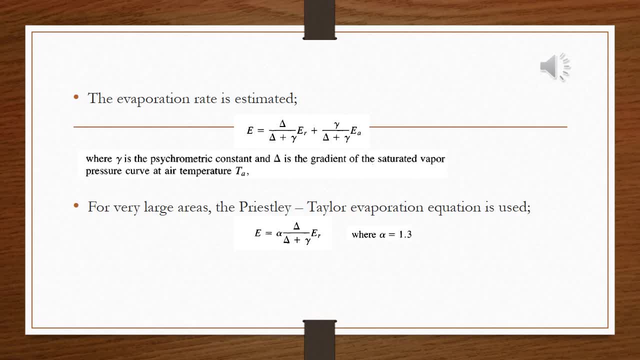 The evaporation rate is estimated. E is equal to delta over Delta plus gamma, Plus the radiation Of like energy balance, Which we take the evaporation Rate in energy balance, Then plus gamma Over delta plus gamma, Which is Aerospace model evaporation Rate is Added. so when we 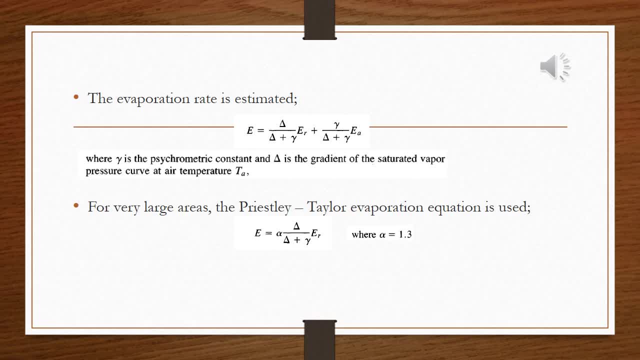 Use this Two equation, Two parameters, We are gonna obtain the Combined method Evaporation rate. Here gamma is the psychometric Constant And delta is the Gradient of the saturated Vapor pressure curve At air temperature. Ta. For very large areas The presley taylor Evaporation equation is used. 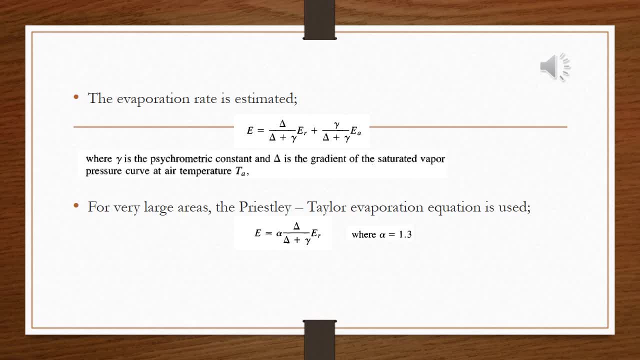 Just like energy balance Equation with the, With the One ratio which is Alpha, Which is taken generally, 1.3, 1.3 multiplied by Gradient of saturated Vapor pressure Curve at air temperature Over again delta plus Gamma, which is psychometric Constant. we need to multiply. 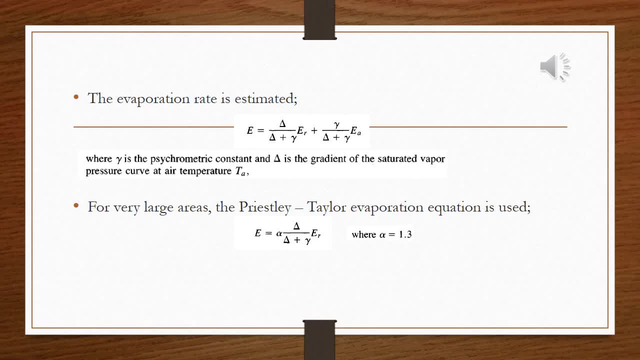 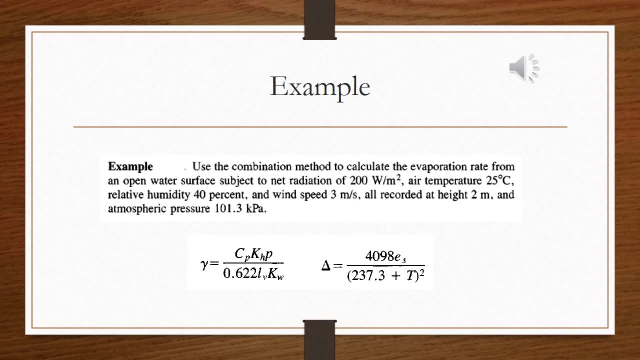 This one with the, Which is, as we See in the Energy balance Rate, The energy balance Or radiation Only, the radiation Evaporation Rate. Okay, We are gonna use The previous example For the Energy balance Method. example: The temperature: 25 Centigrade degree. Relative humidity: 40. 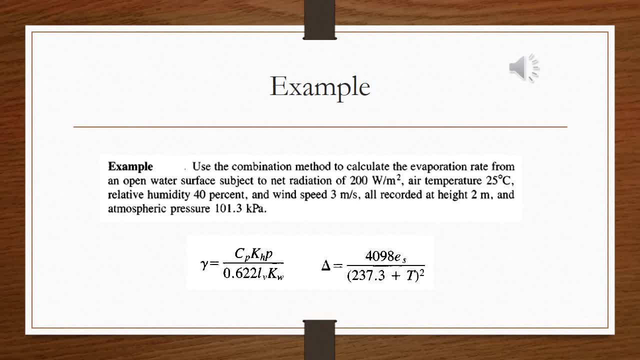 Wind speed 3 meter per second. All recorded height is 2 meter And atmospheric pressure 101.3 Kilopascal Is the same thing We just gonna go through And then we are gonna find ER and EA For energy balance, Equate method, Evaporation rate. 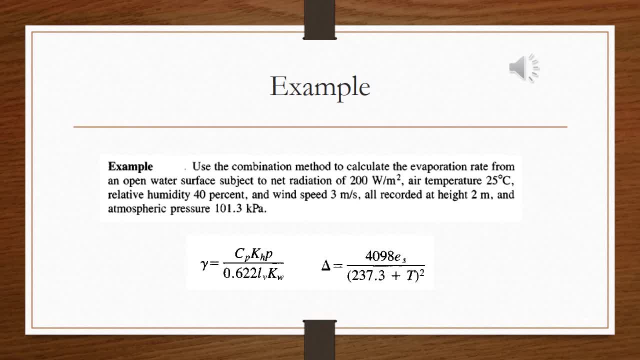 And everything We need to define. first, Gamma and delta. Gamma is Cp, kh, P over 0.622, The latent heat and kw. We are gonna find this Ratio kh over kw. And For delta, we are gonna find We are gonna use 4900 E8 es. 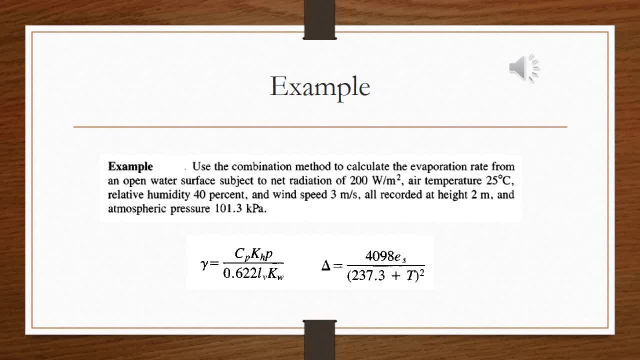 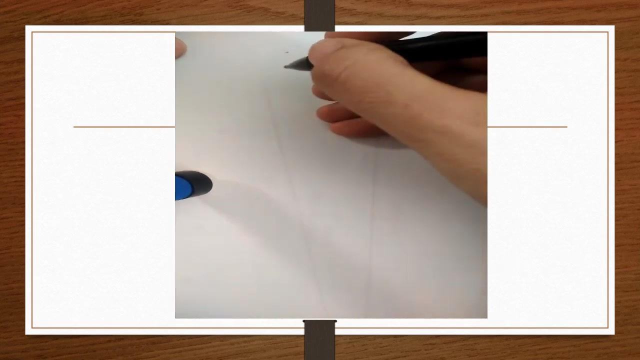 The saturated vapor Pressure, 237.3 Plus temperature Square. Let's go through the example And then I will define This gamma and delta, And we can solve Our New evaporation Rate By using combination method. Okay, Let's First of all start with our Psychometric Constant gamma. 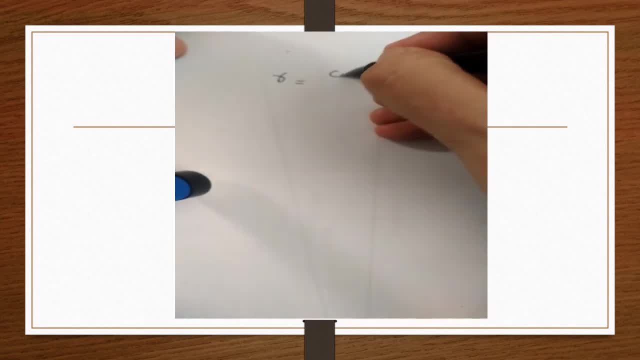 Which is equal to Cp, Kh, P Over 0.622, Latent heat And the kw. So Let's define all of this one: Cp is For air, we are using 1005 For constant pressure, The Specific heat, Let's say Joule kilogram kelvin. 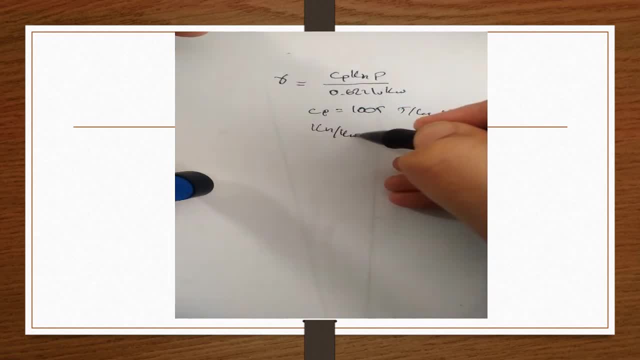 Okay, Kh over kw, Which is this heat. diffusivity Is taken one generally, So This ratio is taken one And The other one is The latent heat at 25 centigrade degree. We already calculated previous example. So it was 2440, So it was 2441. 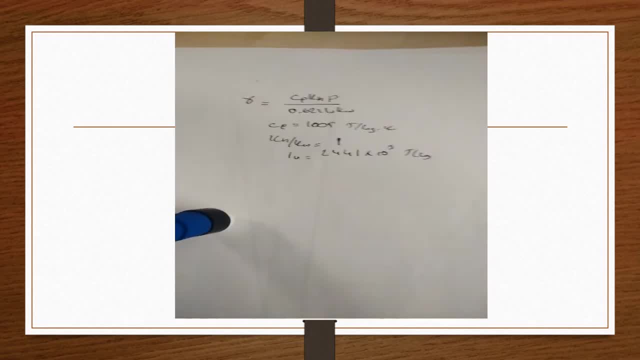 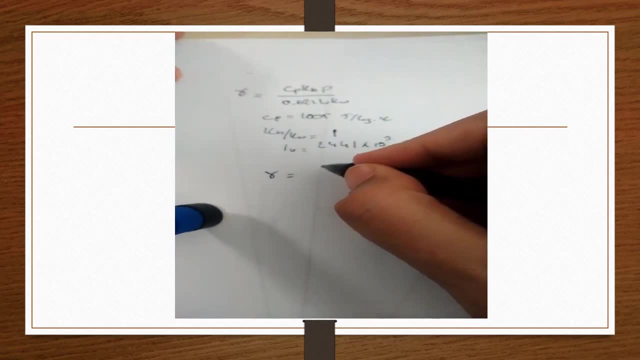 Times 10 to 3 joule over kilogram, Right, Okay, So let's define all of them. Gamma is equal to Cp is 1005, 1005 Kh over kw. I am just writing here one, So I just Take the ratio. We Know that The pressure is. 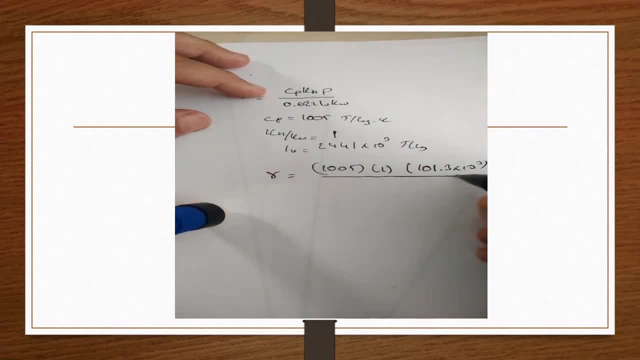 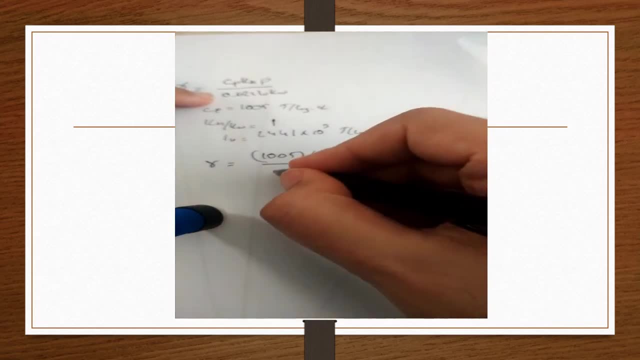 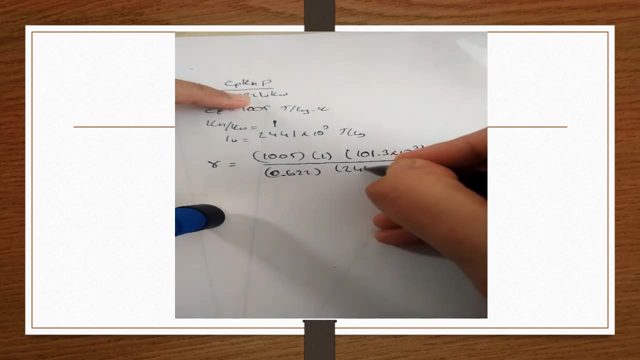 0.3 times 10 to 3 pascal Over. Let me Do it like here: Okay, Over 0.622, And We are gonna write our latent heat, Which is 2441 times 10 to 3 joule over Kilogram At the end. 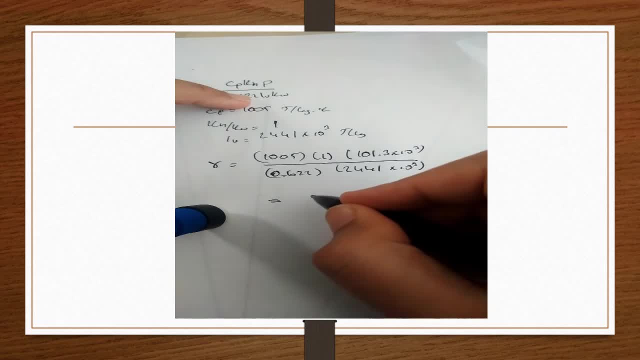 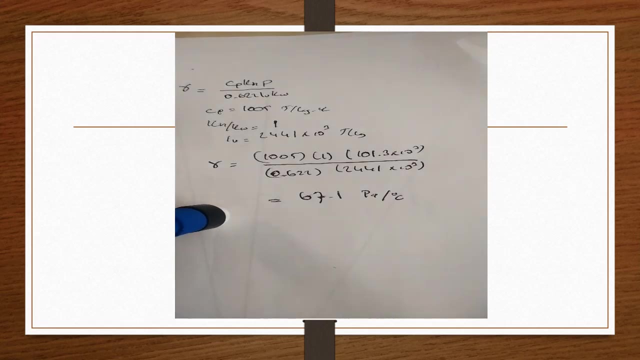 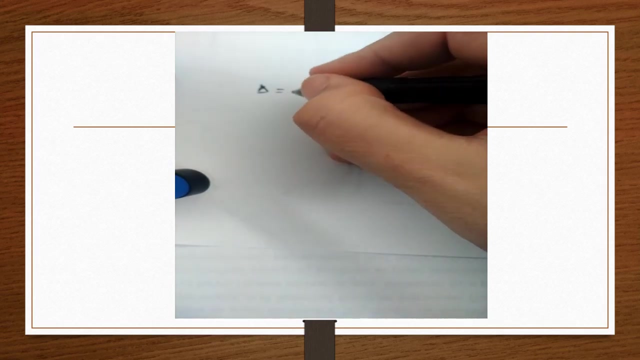 We are gonna find Here Is 67.1, 67.1 pascal Over centigrade degree. So this is For gamma. Let's go through the Define delta For Delta, This gradient Of the saturated water pressure Curve At 25 centigrade degree. It's defined. 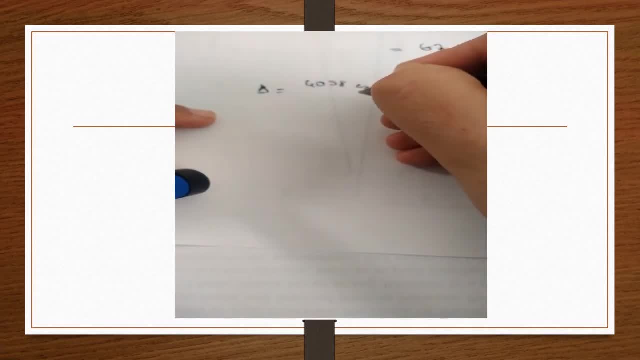 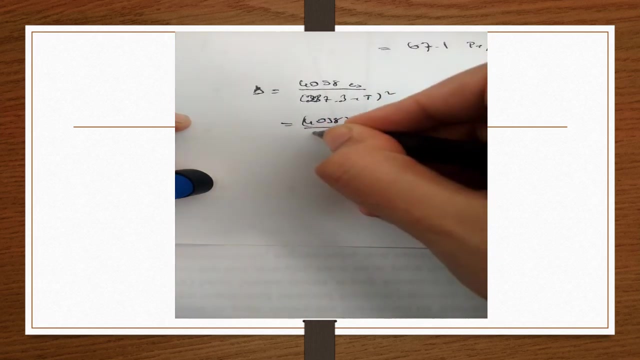 4098 ES, Which is EAS- same thing Which we already defined- Over, Which is saturated. Vapor pressure: 230, 237.3 Plus Temperature square: Okay, 4098, And Let's Define 3167 pascal, 3167 pascal Over 237.3. 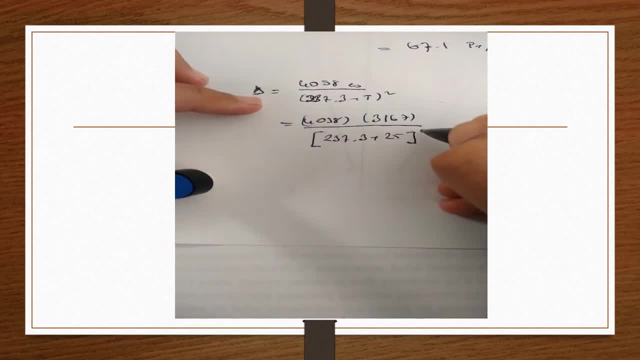 Plus Temperature is 25 centigrade degree Square, And If we calculated, This guy is 188.7 pascal Over centigrade degree. Let's combine all this one And then let's go To our final equation. Let's see. So what was it? E is equal to: 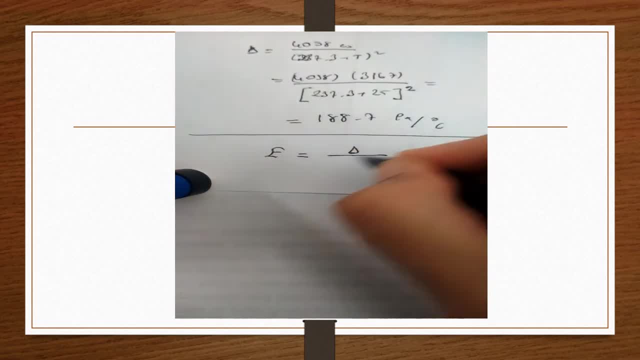 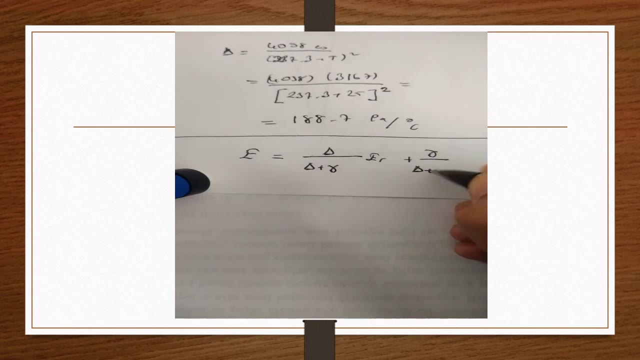 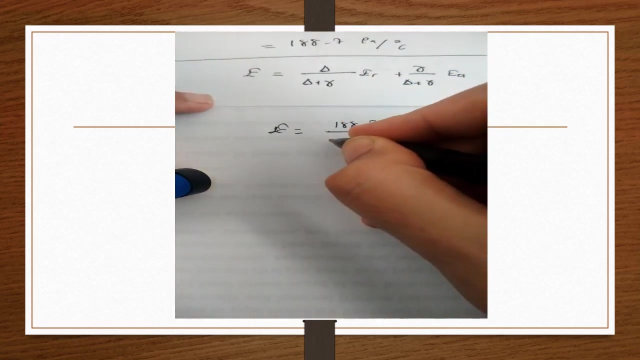 Let's see delta: Delta over Delta plus Gamma From Energy balance Operation rate plus Gamma Over delta plus Gamma From Aerodynamic rate Operation rate. Okay, So E is equal to Gamma is 188.7 Over 188.7 Plus 67.1. Okay, Multiply by: 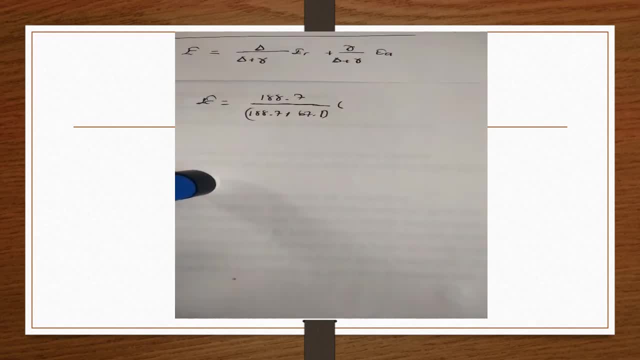 E R. What is E R E R We found? Let me have Here E A. I found Here E R, Here E R. I found 7.1 Millimeter per day, Right, 7.1 Millimeter per day, Right Plus. I am gonna do, I am gonna do.